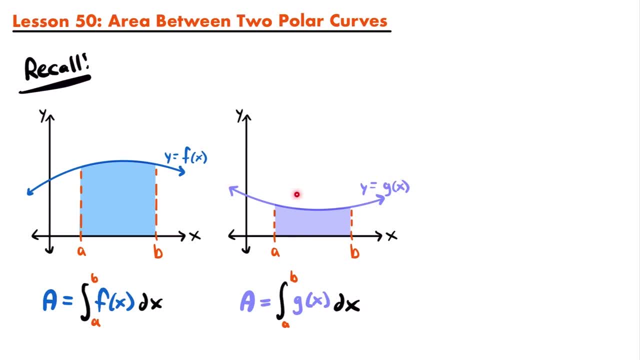 terms of x. We could also calculate the area beneath this curve from a to b using a definite integral. The area is equal to the integral from a to b of g, dx, And so we can calculate the area beneath each of those curves separately. but then, if we put these two curves on the same graph, what we can 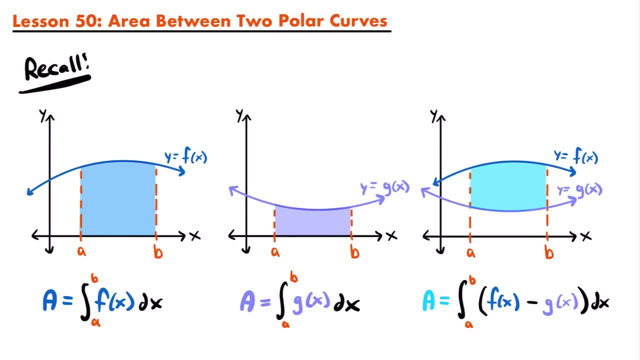 then do is calculate the area between those two curves, that lies between those two values of x, a and b, And we calculate that area using this definite integral, the integral from a to b of f minus g, dx. Alright, and essentially what we're doing here is we're taking the area beneath f and 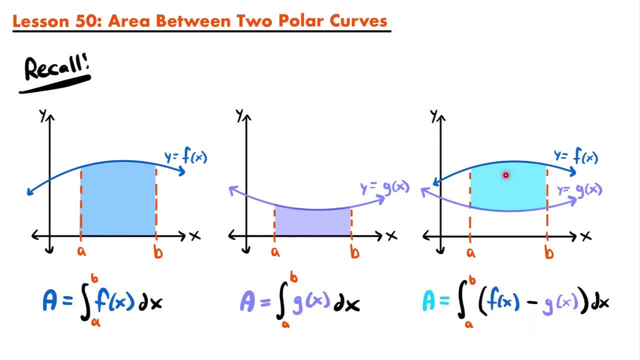 we're subtracting the area beneath g of x to get the area between the two curves Right. the area beneath f of x, that's this area right here. that would be everything beneath this curve. but notice that the area between these two curves does not. 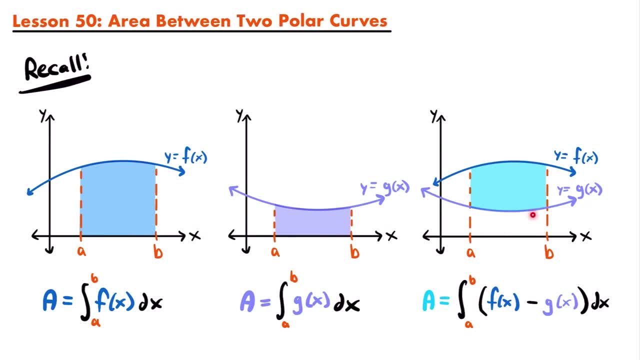 include this area beneath g of x, And so that's why we subtract the area beneath g of x from the area beneath f of x. If we subtract this area from this area, we are left with this area, And so that's what we're doing in this definite. 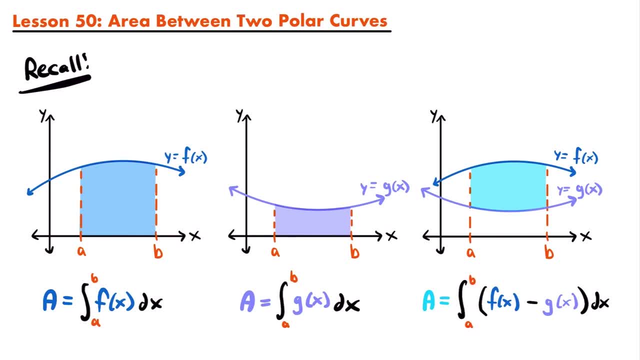 integral. Alright, so this is how we calculated the area between two curves in the rectangular coordinate system, But now what we want to do is apply this same concept to the polar coordinate system with polar curves, And so if you take a look at this graph right here, you can see that we are now working. 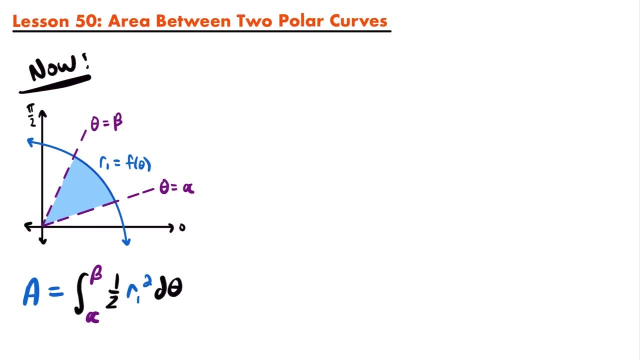 in the polar coordinate system, Our horizontal axis is now the polar axis. we have an angle of 0 right here and we also have our vertical axis- Okay, so this is our integral here- and where the angle is pi divided by 2.. And in this polar coordinate system we have 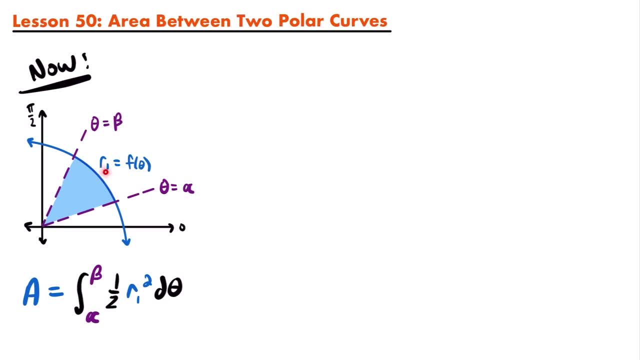 a curve. a polar curve represented by r sub 1 equals f of theta. The radius of the curve is defined by a function in terms of theta And we can calculate the area beneath that curve, between two angles of theta. theta equals alpha, and. 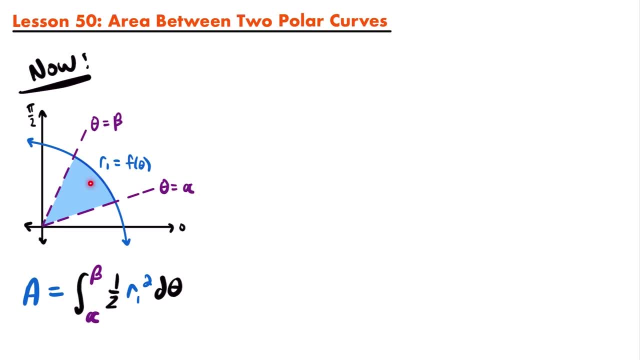 theta equals beta using this definite integral, This area right here is equal to the integral from alpha to beta of 1 half times r sub 1 squared d theta. Alright, and so if you're not familiar with this formula of calculating the area beneath one polar curve, be sure to watch my previous lesson on that topic. 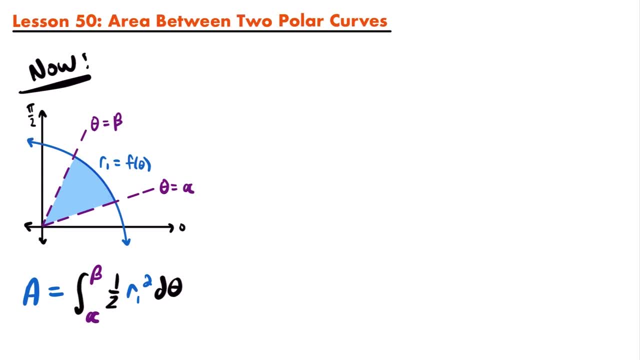 But this is how you can calculate the area beneath a single polar curve, And we can do this for a second polar curve as well. Here we have another polar curve. This time the curve is represented by r. sub 2 is equal to g of theta, So we have 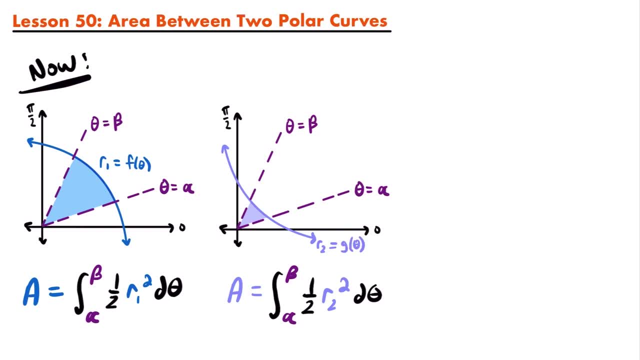 a different curve where the radius is defined with a different function in terms of theta, But we're still calculating the area beneath the curve between the same angles of theta. theta equals alpha and theta equals beta, So we could calculate this area right here using this definite integral. The area is: 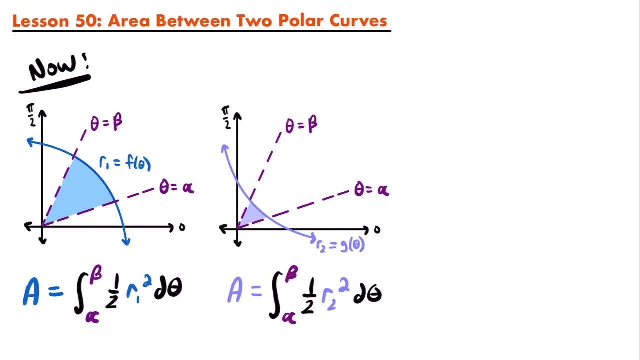 equal to the integral from alpha to beta of 1 half times r sub 2 squared d theta. All right, so in both cases we just have the integral from alpha to beta of 1 half times the function that represents our curve squared, and then we multiply. 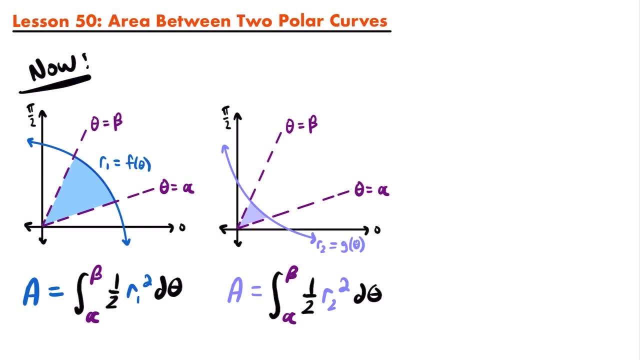 by d theta, theta, And so this is nothing new. We know how to calculate the area beneath one polar curve. The question is, how do we calculate the area between these two curves if we put them on one graph? And so here's what that looks like Here, in this polar coordinate: 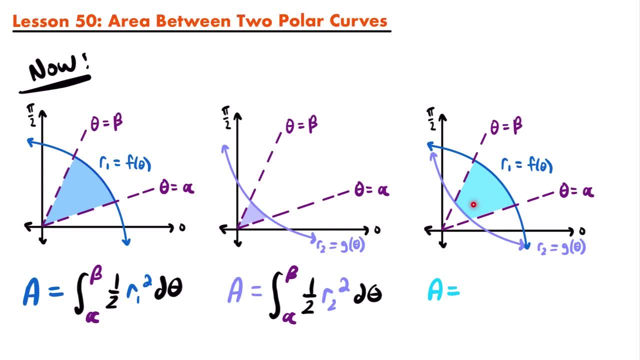 system. we have both of our polar curves and we want to calculate the area between those two curves. that also lies between two specific angles of theta: Theta equals alpha and theta equals beta. How could we calculate this area? Well, the process is very similar to 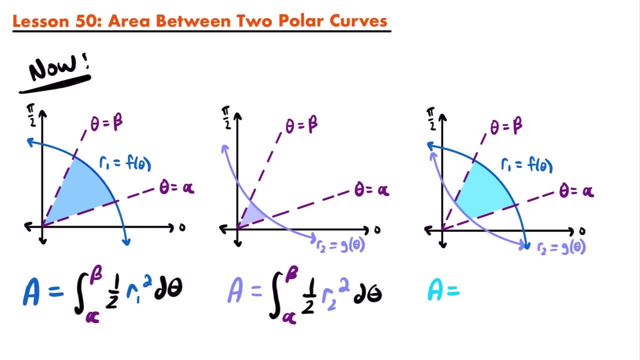 how we do it in the rectangular coordinate system. We can take the area beneath the top curve and subtract the area beneath the bottom curve right. If you take a look at the area beneath each of these curves, this area beneath the top curve would be all of this area right here, and so if you take that area and subtract, 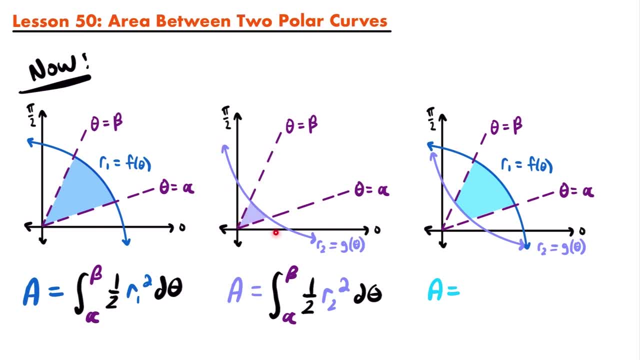 out this little bit of area beneath the lower curve. that will remove this area that is no longer shaded in here here, and you'll be left with the area between the two curves. So what we can do is subtract this area from this area So we can represent the area between the two polar curves with. 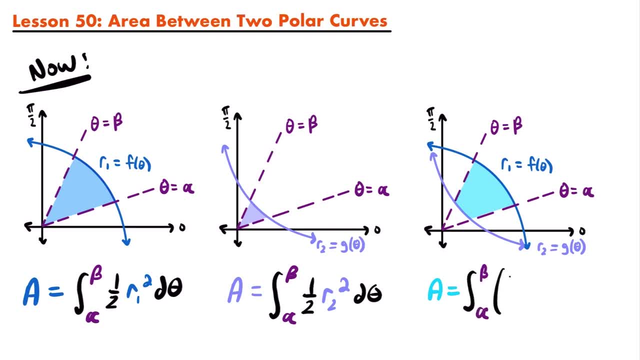 an integral, from alpha to beta, of one half times r sub one squared minus one half times r sub two squared times d theta. Alright, so all we did there was combine these two definite integrals by subtracting this integral from this integral, Since both of these definite 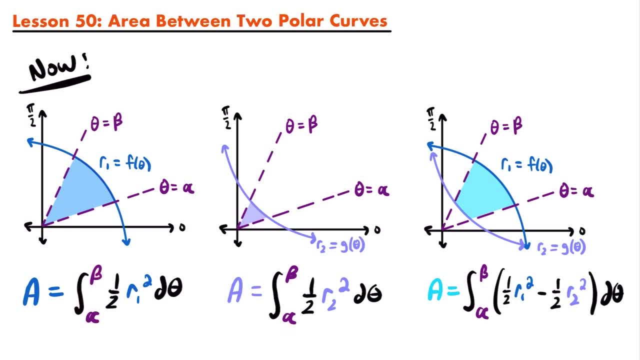 integrals have the same bounds of integration of alpha and beta. we can combine them by subtracting the second from the first, And that is exactly what we have right here. Alright, and so this definite integral, if you know the two polar equations that represent your polar curves. 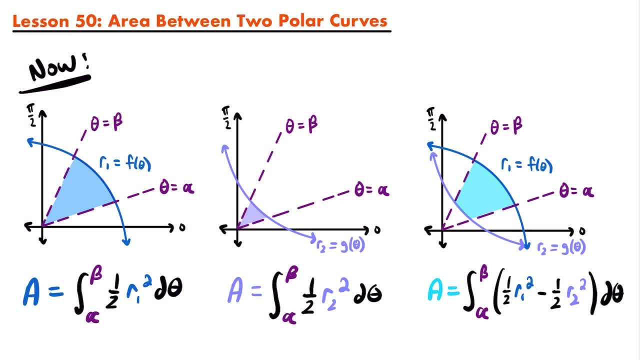 you can plug those into this formula and calculate the area between the two curves. Now you can simplify this definite integral a little bit. Both of these terms have a common denominator of one half that could be pulled out to the front of the integral, So you could have one. 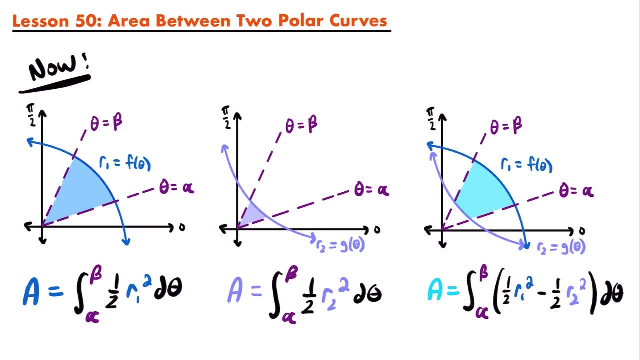 half times the integral from alpha to beta of r sub one squared minus r sub two squared. And then you could also rewrite r sub one and r sub two to be their respective functions in terms of theta, So you'd have f of theta squared minus g of theta squared. And so if 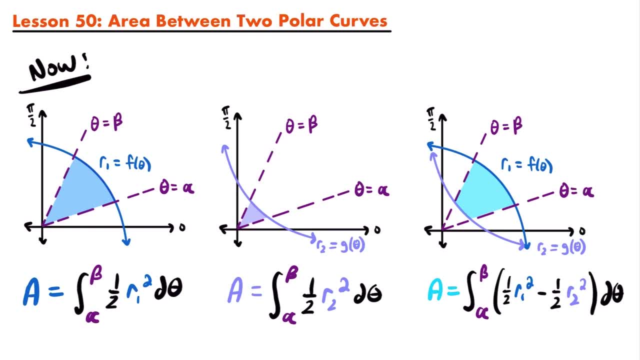 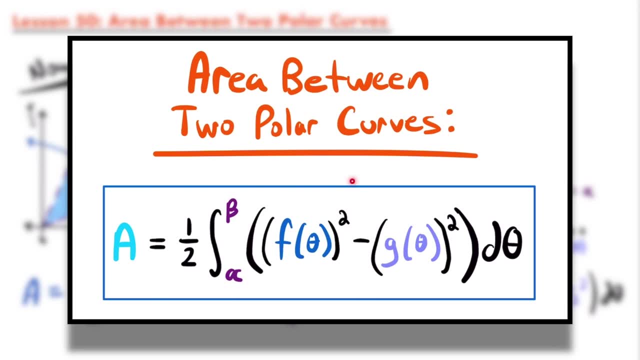 you wrote the definite integral like that, you would get the general form of the integral that calculates the area between two polar curves, And that definite integral looks like this: The area between two polar curves can be calculated using this definite integral, which is that the area is equal to one half times the integral from alpha to beta of f. 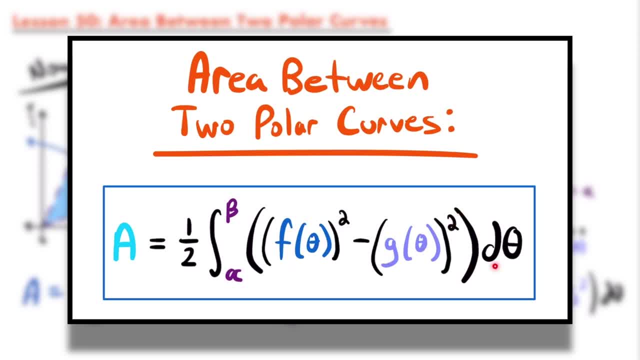 of theta squared minus g of theta squared times d theta. Alright, so f of theta represents the outside curve or the top curve of the area that you want to calculate. You can think of f of theta as being the curve with a bigger radius, And then g of theta represents the. 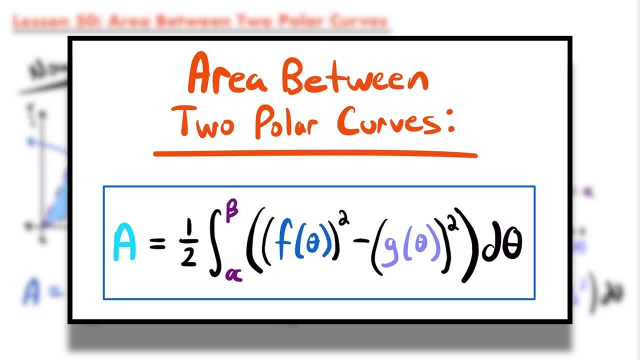 inside curve, or the lower curve or the upper curve of the area. you want to calculate the curve that bounds the area at the bottom, or you can think of g, of theta, as being the polar curve with a smaller radius. Alright, so in general, for most cases where you want to calculate the area between two, 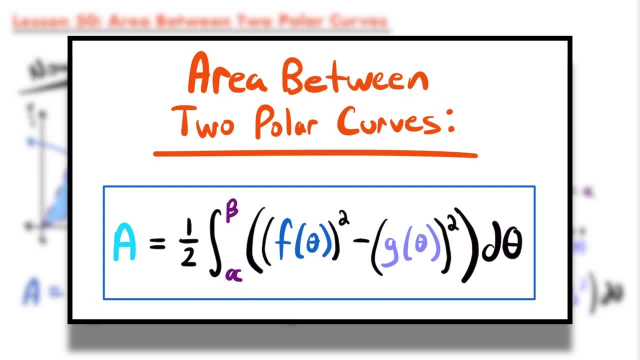 polar curves. this is the definite integral that you can use to calculate that area. But now, before we look at an example of using this definite integral, I do want to make it clear that this definite integral is not going to apply in every single scenario where. 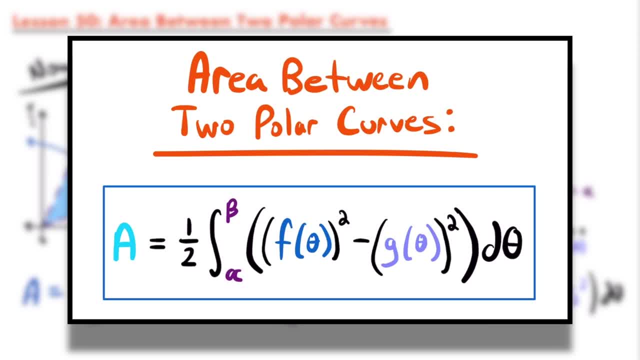 you want to calculate area bounded by two polar curves, This definite integral will work in a majority of problems, but there are going to be certain problems where you want to calculate the area of a shared region between two polar curves and in those cases this definite integral will not be applicable. 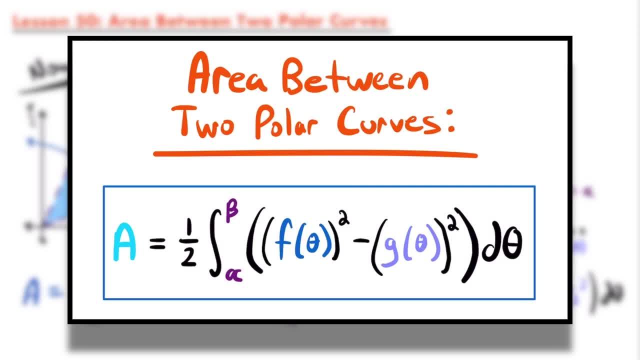 You're going to have to think a little bit more intuitively on how to calculate the area for that particular problem, And we'll take a look at an example of that in this video. but first I want to take a look at a basic example. 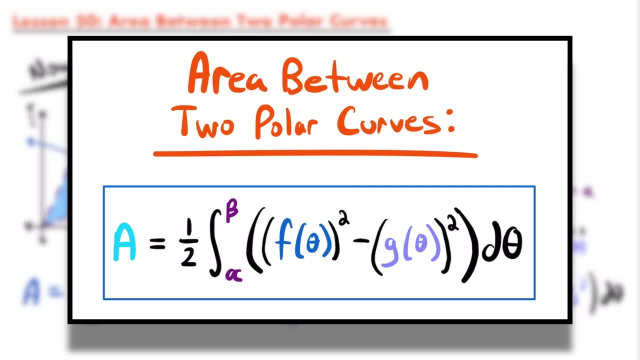 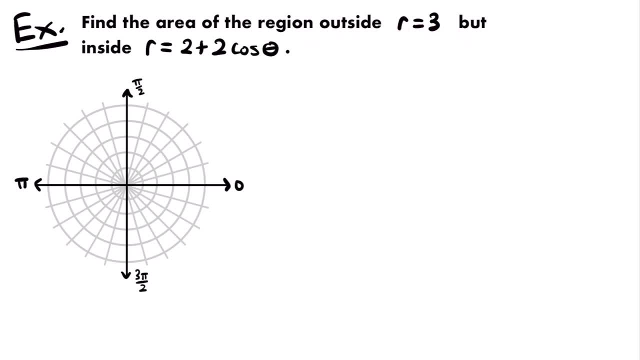 Where this definite integral will work. And so let's take a look at that next. Alright, so here's our first example. We want to find the area of the region outside r equals three, but inside r equals two plus two times cosine theta. 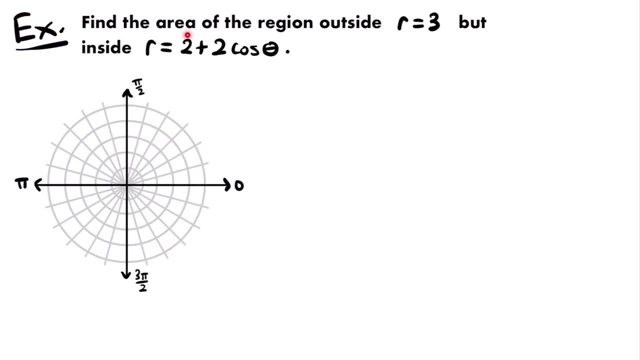 And so the first thing that I always recommend that you do when you want to calculate the area between two polar curves, is first draw a graph of that area. And so let's graph each of these polar curves. I'll start by graphing: r equals three. 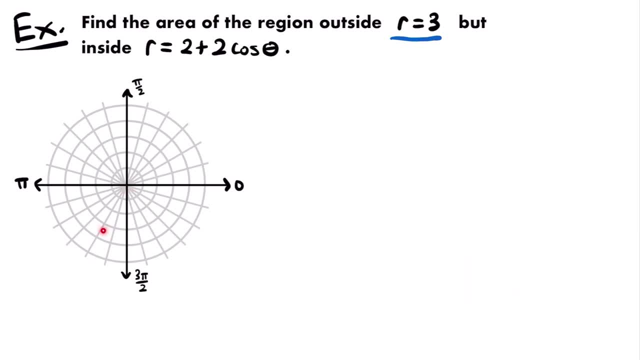 R equals three is just a circle. This is centered at the origin of the polar coordinate system, where the radius of that circle is three. So if each of these circles represents a unit of one for the radius, then this first circle is a radius of one, the second circle is a radius of two, and then we have three, four. 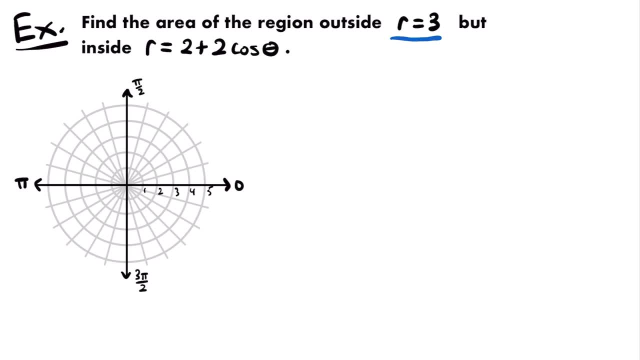 and five, So a circle centered at the origin with a radius of three will look something like this: Alright, we have a circle centered at the origin that rests along the concentric circle where the radius is three, And then let's graph our circle. 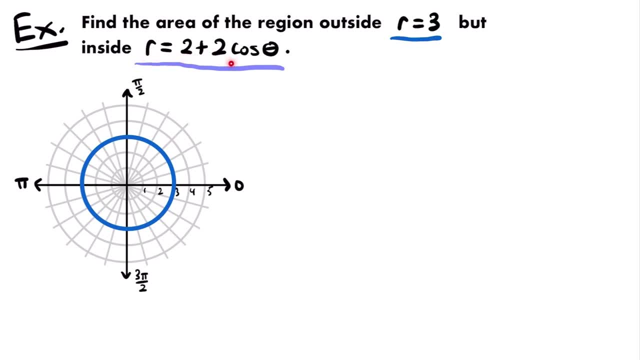 Let's graph our second polar equation. here We have: r equals two plus two times cosine, theta, And hopefully by this point you are familiar with your special types of polar graphs. This polar equation right here, since you have a constant plus a constant times cosine. 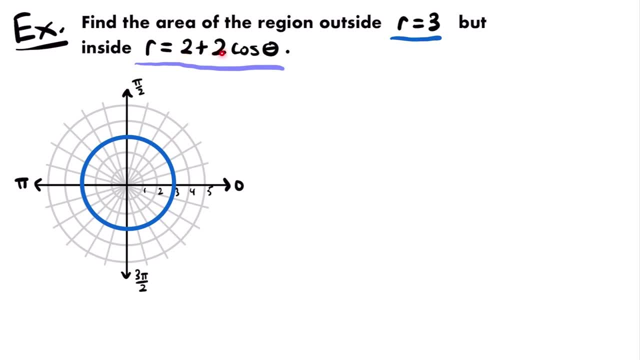 theta. you know you are working with a limousine And in this case both the constants are the same, And when they are the same, you know you're working with a cardioid And so the basic shape of a cardioid. when you're working with cosine theta instead of 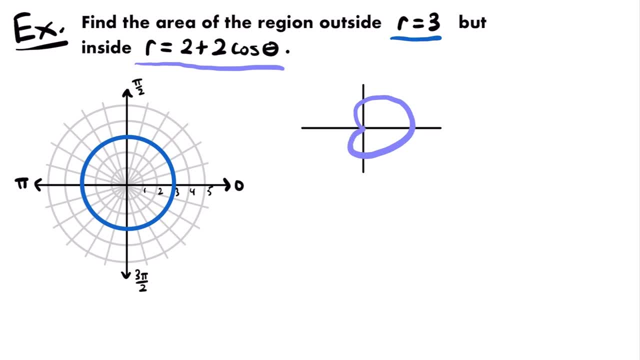 sine theta. is this shape right here? Okay, So if the form of a polar equation that represents a limousine is: r equals a plus or minus b times cosine theta, then we can use those values of a and b to determine where this cardioid will be in our polar coordinate system. 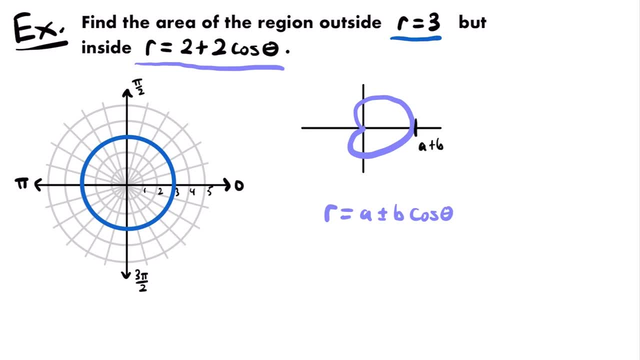 Specifically, this back end is a radius of a plus b and the cardioid crosses through the vertical axis at a, above and below the polar axis. Okay, so in this case, our value of a is two and our value of b is two. So a plus b is equal to two plus two, which is equal to four. 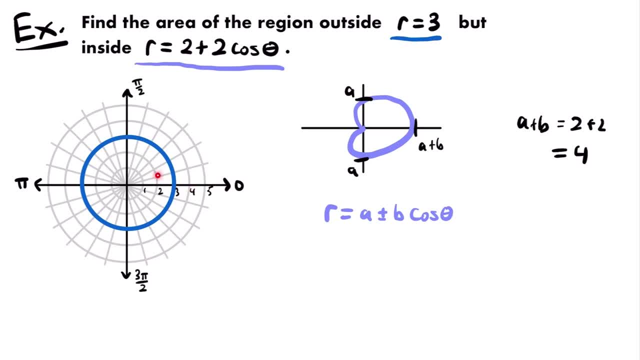 So the back end of our cardioid will be at a radius of four and our value of a is two, So the cardioid will cross through the radius of two above and below the polar axis. So if we graph our cardioid, it will look something like this: 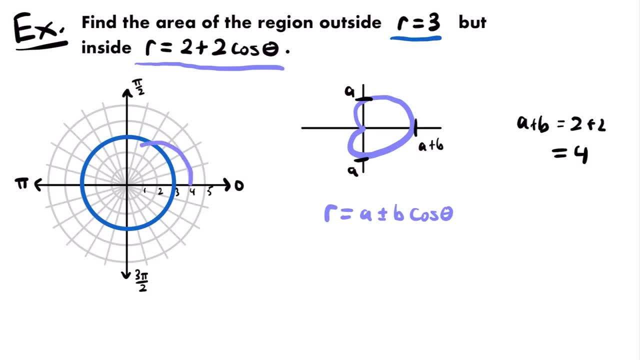 We'll start at the back end, where the radius is four. We'll come through, cross through the radius of two along the vertical axis, hit the origin, come back out, cross through two again and then come back to our radius of four. 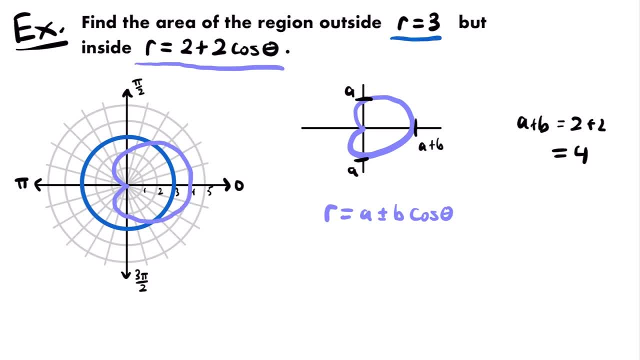 Okay, Okay. So that's not a perfect drawing of our cardioid, but it's good enough for us to see the area that we're going to calculate. All right, So now what we can do is determine what area we are trying to find. 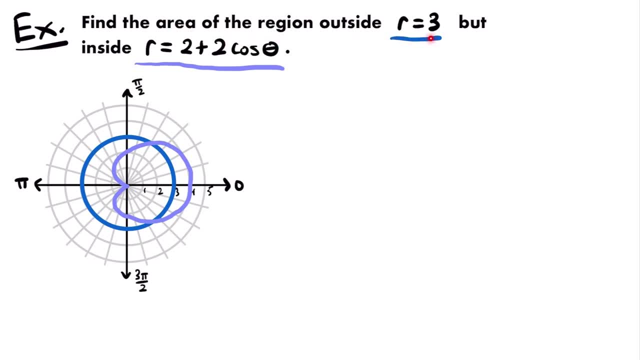 We want to find the area of the region. outside r equals three, but inside r equals two plus two times cosine theta. So outside r equals three means that we are not going to be calculating any area within the circle, We are going to be calculating area outside of the circle. 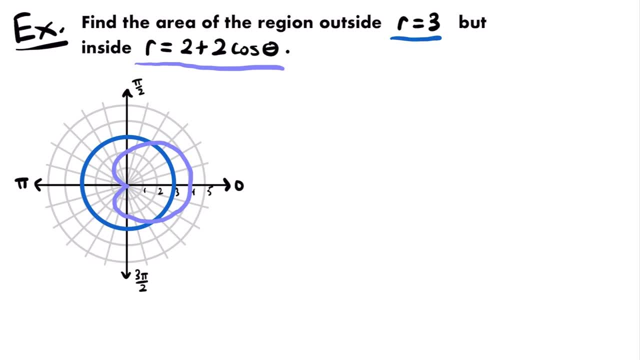 That is also inside the cardioid, And so, if you take a look at our graph, the only area that meets those requirements is this little crescent shape right here. This area is within the cardioid, but outside of the circle, All right. 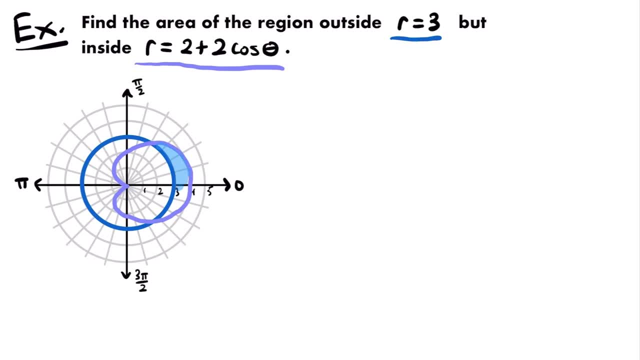 And so I'm going to shade that region in. This is the region that we want to calculate the area of, And you can see that it is an area that lies between two polar curves. It lies between this curve, which is part of this cardioid, and this curve, which is part of the region. 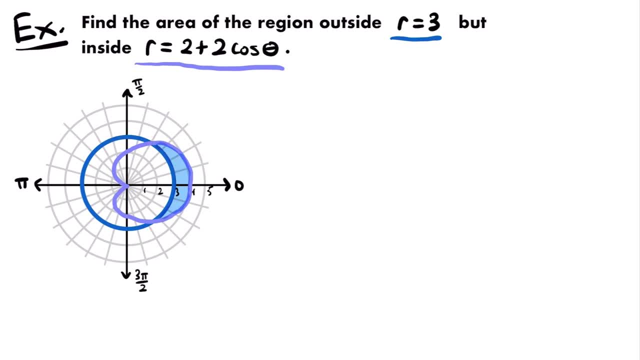 And this is the region that we want to calculate the area of. So we can calculate this area using the following definite integral: The area is equal to one half times the integral from alpha to beta. Those are two values of theta or two angles that are area lies between of f, of theta squared. 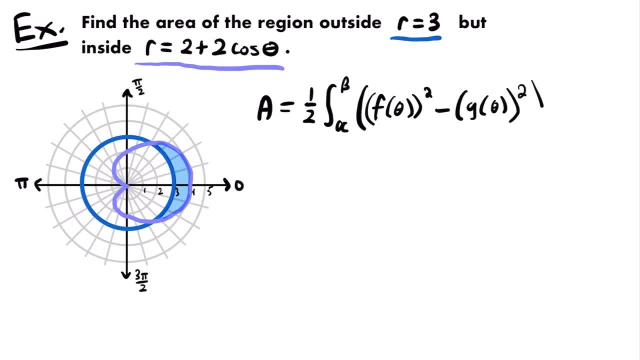 minus g of theta. All right, So we have a couple of things that we need to determine here. We need to decide which of our two polar curves is f of theta And which of the two curves is g of theta. Remember that f of theta is the outside curve, or the curve with the bigger radius. 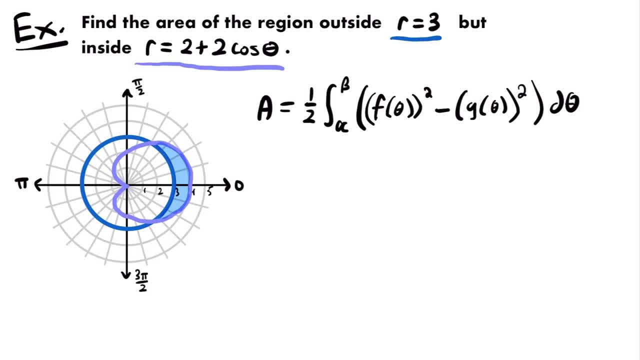 And g of theta is the bottom curve, or the curve with the smaller radius. And so if you take a look at our polar graph here, you can see that for this region the cardioid is on the top part of the region. For this part of our graph, the cardioid has a bigger radius. 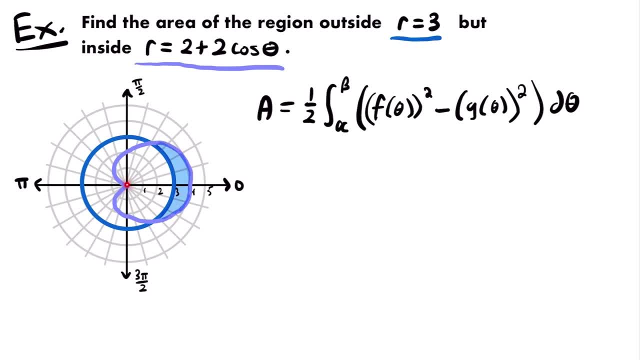 It is further away from the origin, Right? If you're looking at the distance from the origin to this region, The cardioid is the furthest away, It has the biggest radius, And so that means that for this region the cardioid will be f of theta and the circle. 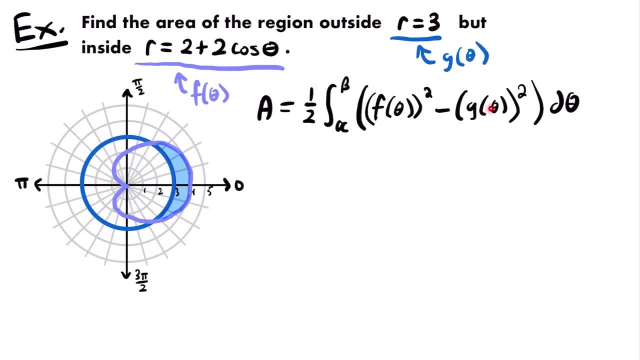 will be g of theta. Okay, So we could plug three in for g of theta and we could plug two plus two times cosine theta in for f of theta and we could square them and then integrate. However, we still need to determine our angles of theta alpha and beta. 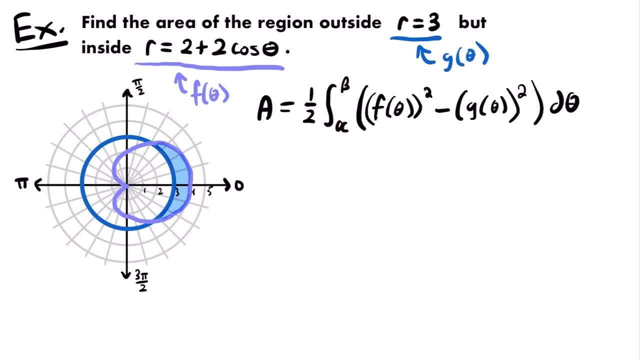 What two angles of theta does this area lie between? And so how do we go about determining those angles? Well, what you can notice is that those two angles are going to occur where these two curves meet. Alright, When these two curves intersect. that is where this area is contained between. 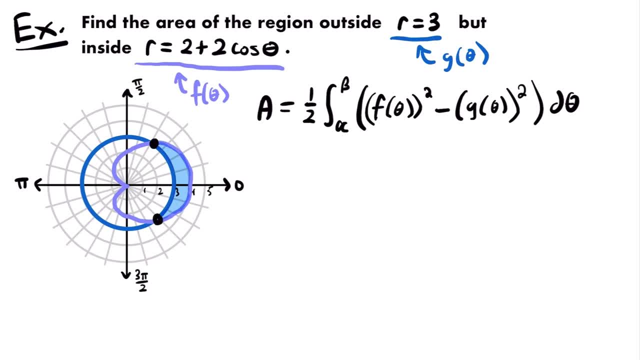 This point right here where the curves meet, and this point right here where the curves meet. So if we can determine what angle corresponds to each of these points, we can determine our bounds of integration. And so to do that, Okay, where these two curves intersect. 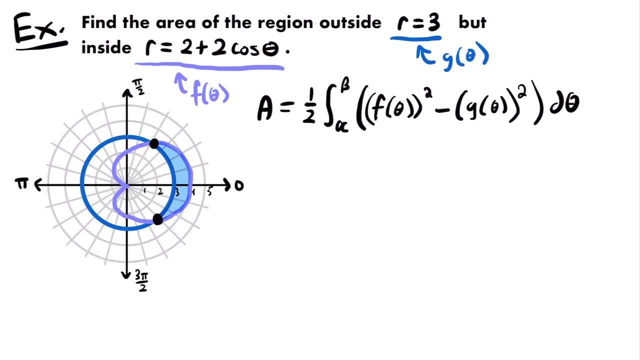 And if you remember from algebra, whenever you want to determine where two curves or two lines intersect, you just set the curves or the lines equal to each other and solve In algebra. you solve for x, but in this case we're gonna be solving for theta. 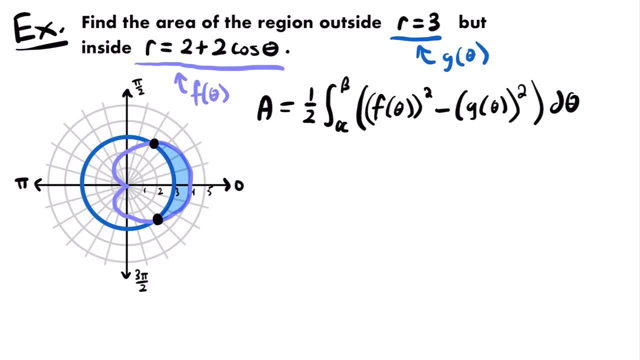 All right. so if we set these two polar equations equal to each other, since they're both equal to r, right, we have: r equals three and r equals two plus two times cosine theta. we can replace this r with three and then solve for theta. 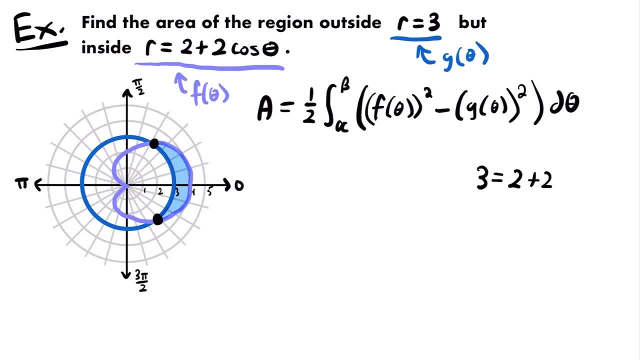 So if I do that, we'll have: three is equal to two plus two times cosine theta. And now what we have to do is solve for theta, and that will give us the angles of the points where these two curves intersect- this point and this point. 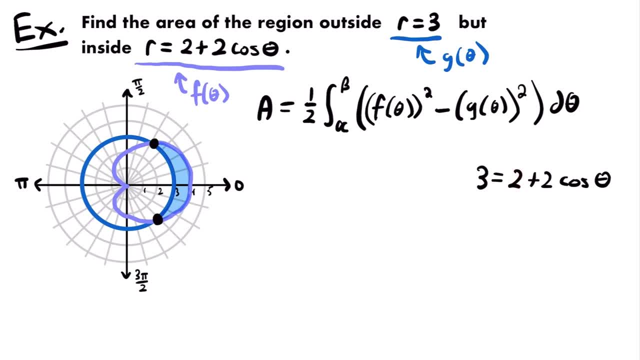 And so let's solve for theta. First thing I'm going to do is subtract two from both sides of the equation, So we'll have: one is equal to two times cosine theta. Then we can divide both sides by two to isolate cosine, and so we'll have 1: 1⁄2 is equal to cosine theta. 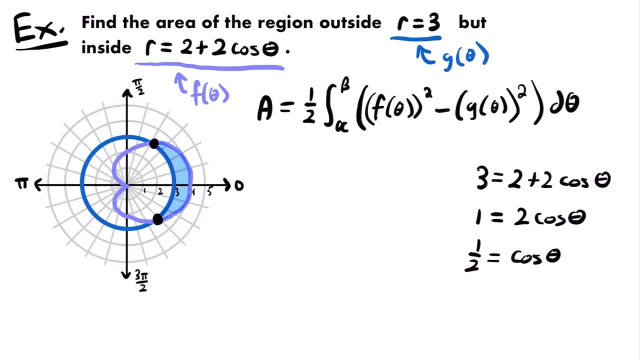 And now, at this point, this should be pretty easy to solve. You just have to ask yourself what angles of theta would make cosine equal to 1 1⁄2. And if you're familiar with cosine, you know that cosine of pi divided by three. 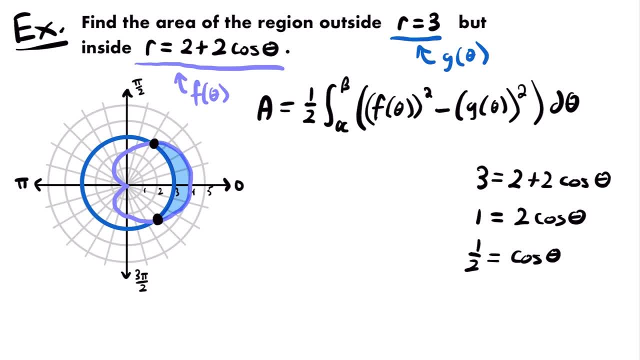 and five pi divided by three are when cosine is equal to 1 1⁄2.. So this equation gives us two angles: theta equals pi divided by three and five pi divided by three, At least if you're working with angles of theta. 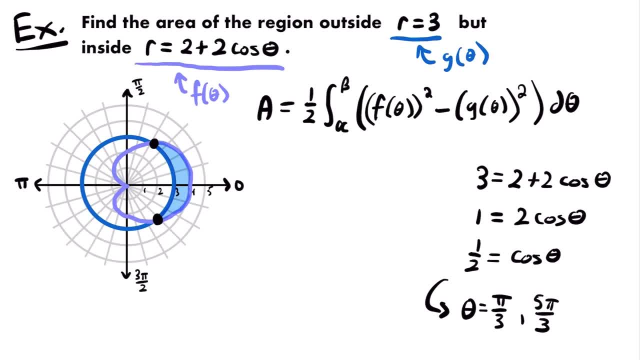 between zero and two pi, like we are in the polar coordinate system. All right, one full circle is two pi. If you look at any angles after two pi, you're just going to be looking at repeated points. So there's no reason for us to look further than two pi. 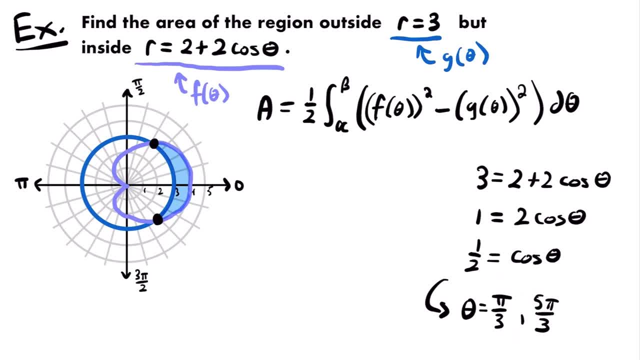 All right. so these are the only two angles where cosine theta is equal to 1 1⁄2 in this scenario, And so theta equals pi divided by three. That will be this angle right here, right, If you're starting at an angle of zero. 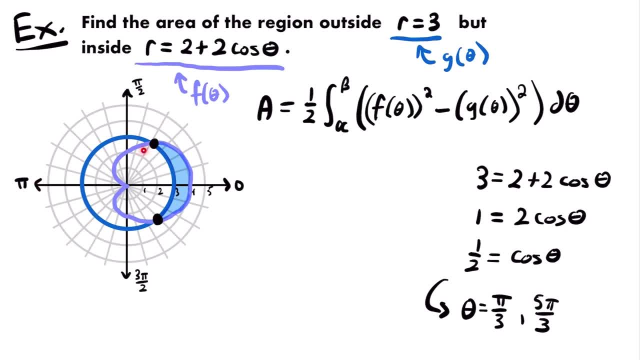 pi divided by three will be a third of the way to pi, So that will be this angle. So I'll label this angle With pi divided by three, And so that means that this other angle of five pi divided by three will be this angle. right here for this point. 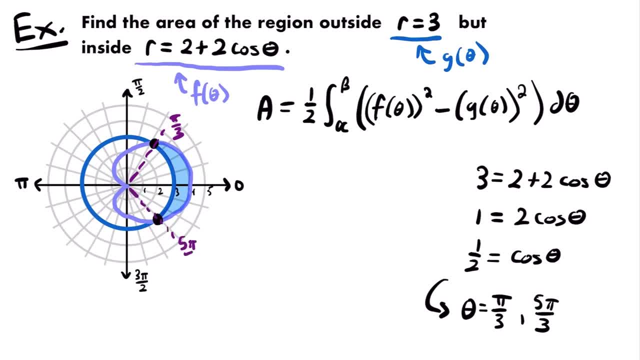 So I'll label that. This angle right here is five pi divided by three. Okay, now, I didn't completely draw this to scale, This angle should probably be closer to three pi divided by two. but don't worry about that, My drawing just isn't perfect. 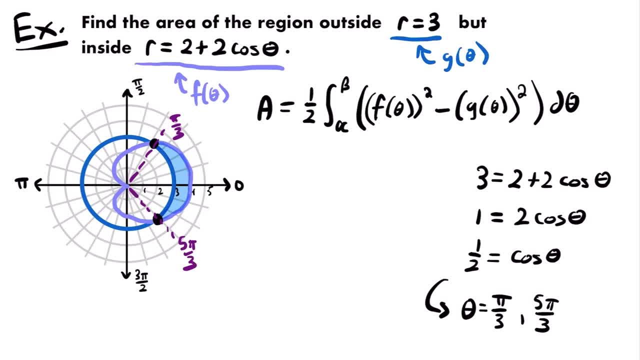 But just know that at these two points where the curves intersect, that the angles are pi divided by three and five pi divided by three. all right, And so now we are ready to set up our definite integral, But we still have to be careful about how we set it up. 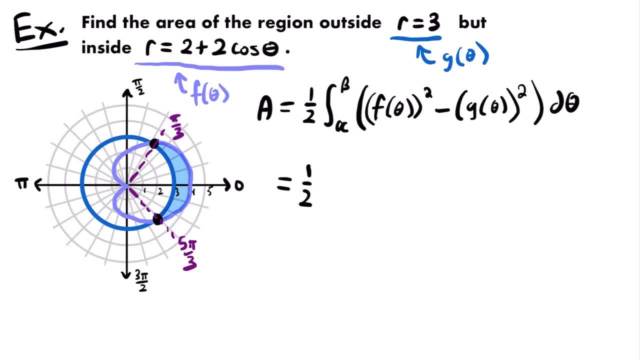 And let me show you why. The area is going to be equal to one half times the integral between two angles of theta that the region lies between. Now you might be tempted to make your lower bound five pi divided by three and your upper bound pi divided by three. 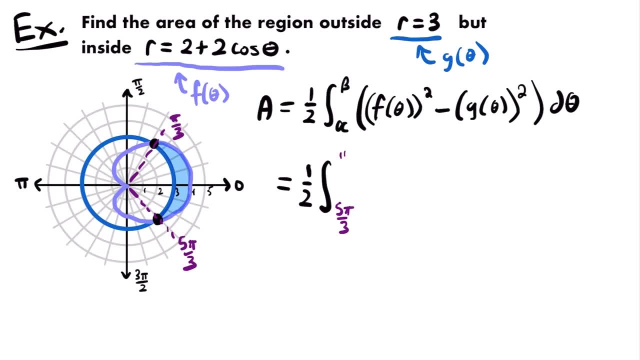 If you were to do that, if we had five pi divided by three and pi divided by three, that doesn't really make sense. Right, We're going from a bigger angle to a smaller angle. We can't do that. It just doesn't make sense. 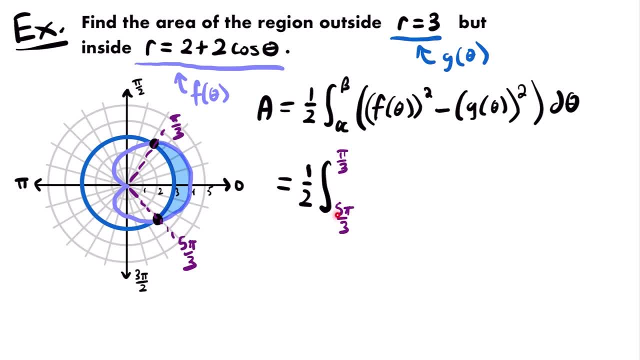 And so then, maybe your next thought is: okay. well, I can't integrate from a big angle to a small angle. so what if I integrate from pi divided by three, the smaller angle to the bigger angle? Well, that's not going to work either, right? 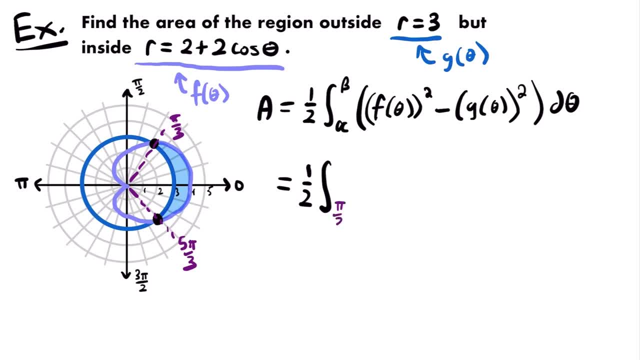 If we rewrite our bounds of integration here and we integrate from pi divided by three to five pi divided by three, if you were to look at the graph over here between those two angles, if we start at this angle right here- pi divided by three- and we increase the angle. 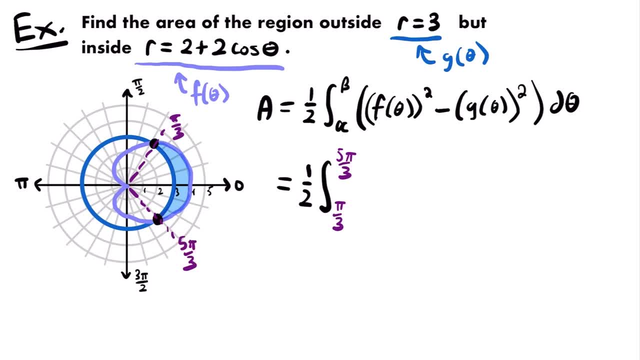 to five pi divided by three. well, we're just calculating a completely different area there, right? We're calculating the area from this angle to this angle, which would be this area right here We don't want to calculate the area between pi divided by three and five pi divided by three. 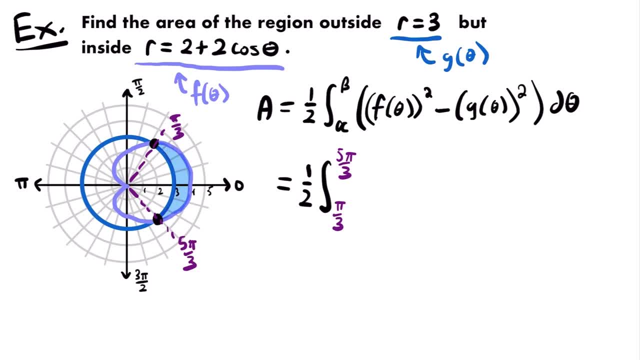 We want to calculate this area right here, And so how can we fix this? How can we set up our bounds in such a way that we calculate the correct area? Well, what we can do is rewrite what five pi divided by three is right. 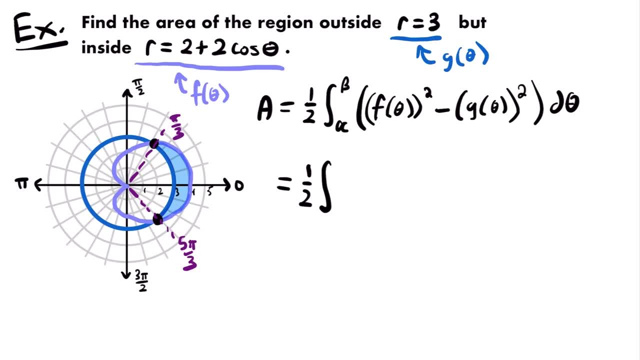 Five pi divided by three is going to be the same as negative pi divided by three. okay, Remember that you can work with negative angles If you start at this angle of zero and you want to measure an angle of negative pi divided by three. 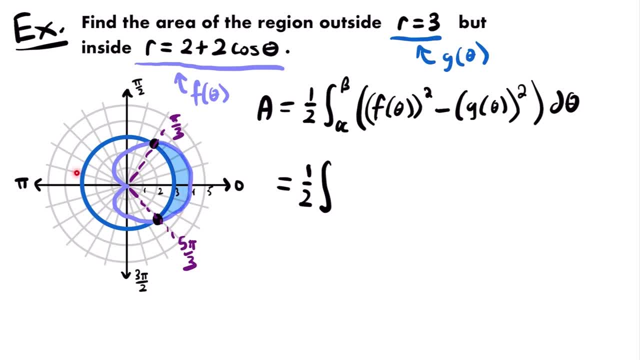 you're going to measure that negative angle by moving in the clockwise direction. Negative pi divided by three will take you to this angle right here. all right, And you could find that by remembering that six pi divided by three is two pi right. 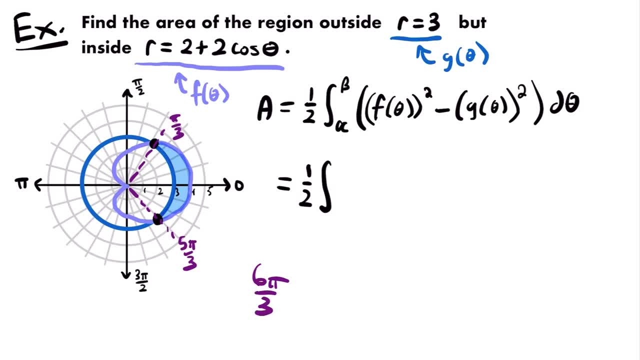 Six divided by three is two. So if you subtract one pi divided by three like this, that will give you five pi divided by three. all right, So negative pi divided by three or an angle of pi divided by three before two pi will take you. 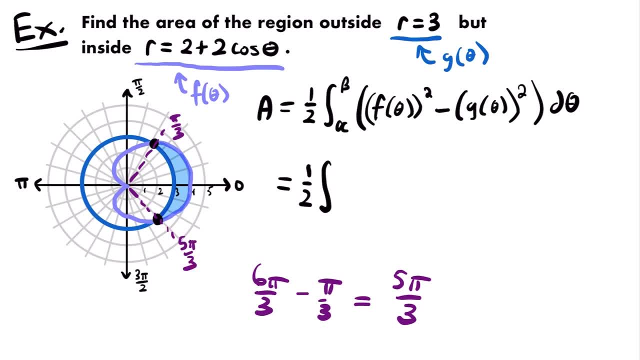 to five pi divided by three. That's the same as negative pi divided by three. all right, So we have five pi divided by three or negative pi divided divided by 3.. Okay, so we can set up our definite integral like this: We'll have a lower bound of. 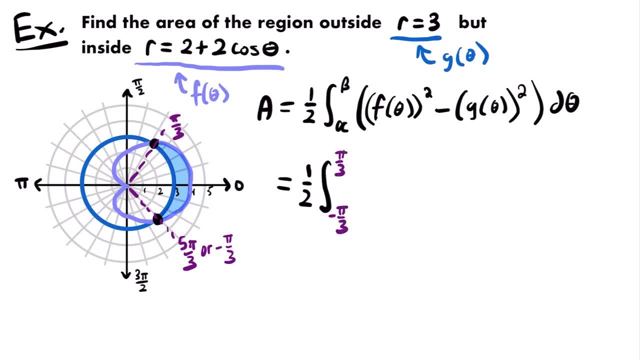 negative pi divided by 3 to pi divided by 3.. We're integrating from a smaller angle to a bigger angle, and the area between those two angles is the area that we want to calculate: From negative pi divided by 3 to positive pi divided by 3.. Okay, so now we can set up the rest of our definite integral. 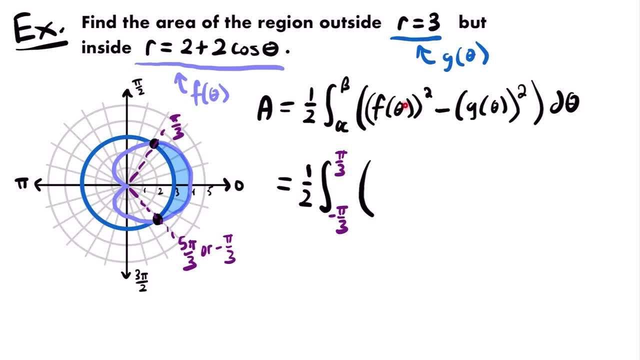 We will be integrating f of theta squared and we determined that f of theta is this equation. So we'll have 2 plus 2 times cosine theta squared, and we will subtract g of theta and we determine that g of theta is 3.. So we'll have 3 squared and then times d theta. All right, and so this: 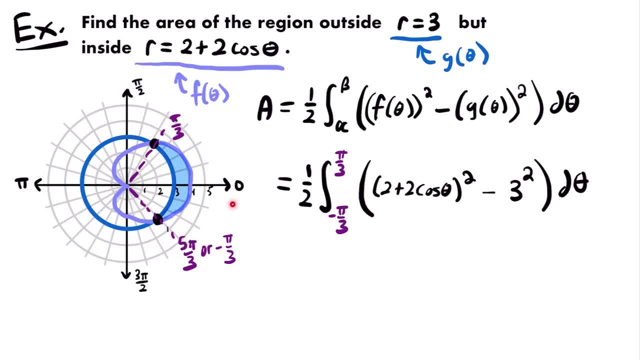 definite integral will calculate the area of this region between these two polar curves. Okay, now, before we go ahead and solve this integral, there's actually one more thing that we can do to make calculating this area a little bit easier, and that is to make this area a little bit easier, and that is to make this area a little bit easier, and that is to make 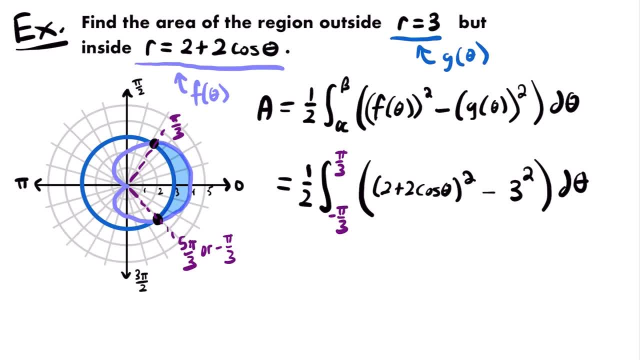 use of symmetry. I made a really big deal out of this when we learned how to calculate the area beneath one polar curve, and I want to stress that same point in this video. when you're finding the area between two polar curves, If you see that you can make use of symmetry to make your integration, 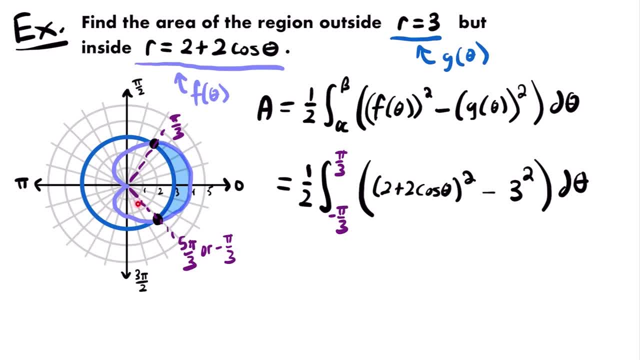 process easier. you should do it In this case. both of these polar curves, this circle and this cardioid are symmetric about the polar axis, which means that this area right here is also symmetric about the polar axis. So we don't have to integrate from negative pi divided by three to pi divided by three. What we can do is integrate from. 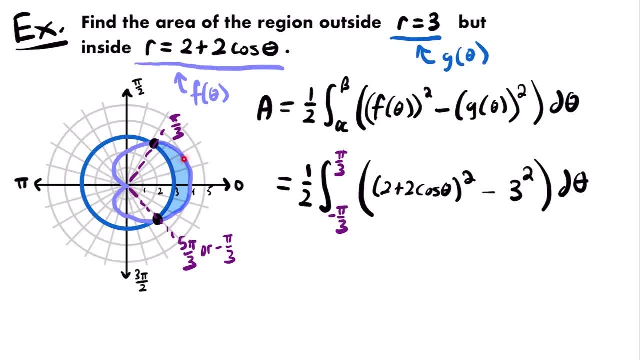 zero to pi, divided by three, find the area of one half of our shape, and then just multiply that area by two to find the area of the whole region. So here's how I will rewrite this definite integral. We'll have that the area is equal to two times, one half times the integral from zero. 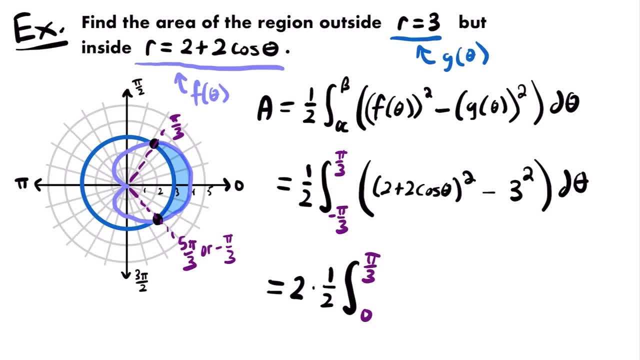 to pi divided by three. All right, so this is just making use of symmetry, which will make our integration process a bit smoother. That way we don't have to work with a negative angle of negative pi divided by three. We can just work with zero and positive pi divided by three. All. 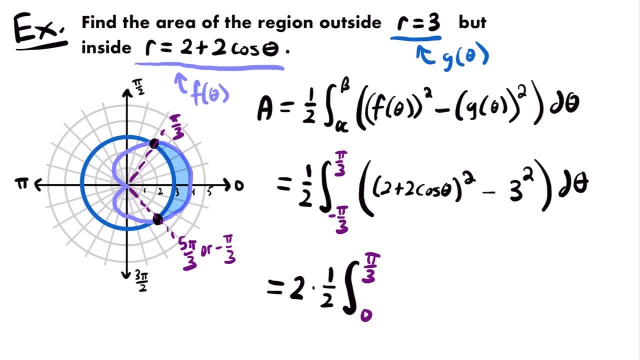 right, and so the rest of the contents of our integral will remain the same. However, I am going to simplify both of these parts. Let's square each of these terms. If we want to square two plus two times cosine theta, we can use a little trick to square it quickly Instead of 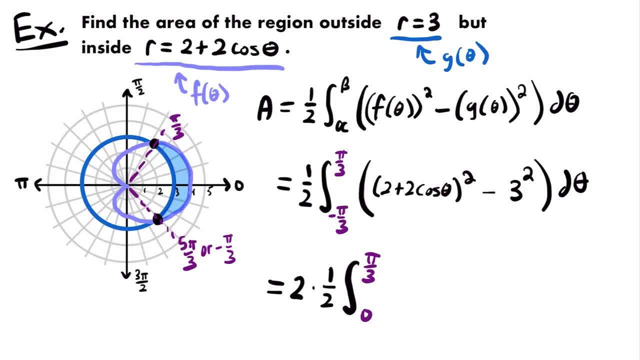 writing out both of these quantities and foiling. what we can do is square the first term, then add these two terms multiplied together, but then multiplied by two, and then add that to the last term squared. So if we do that we'll have four. that's equal to two squared. So we square the. 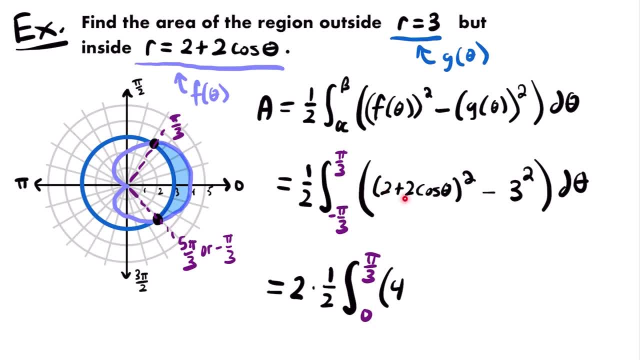 first term. then we multiply these two terms together Two times two times cosine theta is four times cosine theta. But then we need to multiply that by two to get plus eight times cosine theta, and then we'll add that to the last term squared And two times cosine theta squared. 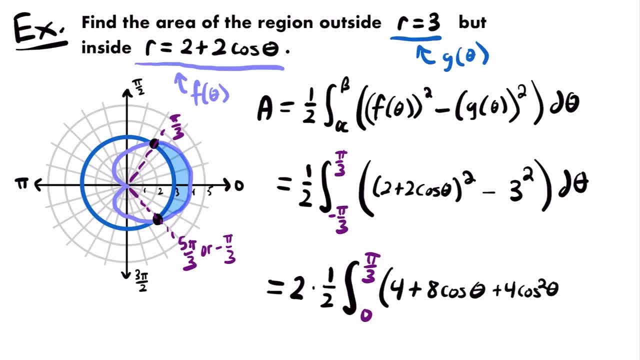 will be four times cosine squared theta. Alright, 2 squared is 4, and cosine theta squared is cosine squared theta. And then don't forget to subtract 3 squared, which is 9.. So we'll subtract 9.. And then don't. 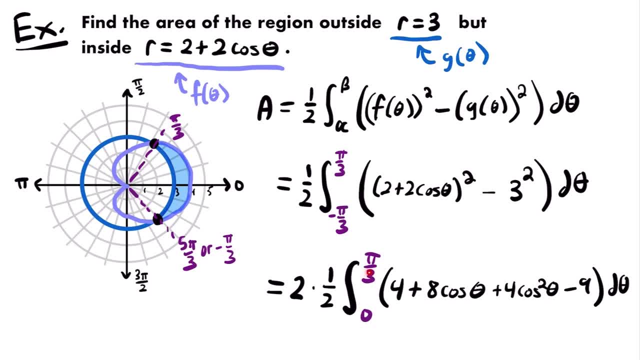 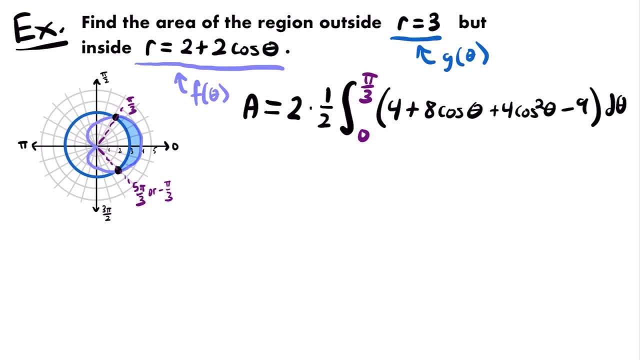 forget d theta. Okay, so now we can solve this definite integral to calculate the area between these two polar curves. Alright, so the first thing that we can do to simplify is multiply 2 times 1 half. That's just going to be 1.. These two constants cancel each other. 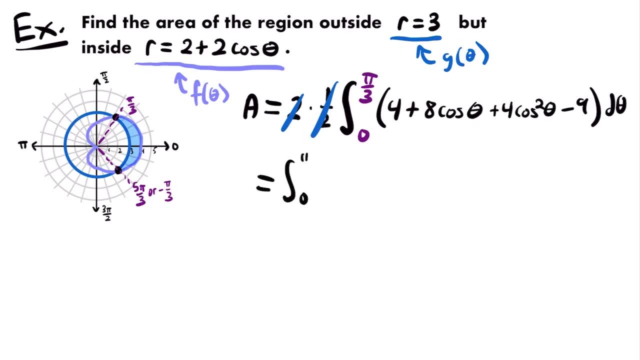 out. So the area is equal to the integral from zero to pi divided by three of these terms. Now we can combine four and negative nine to be negative five. So I'll combine them when we rewrite our terms, But notice that that constant of negative five will be. 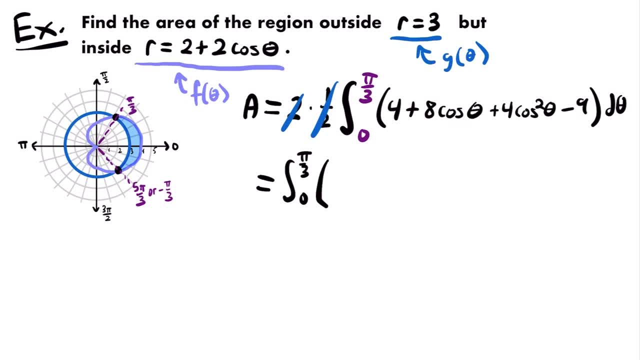 pretty simple to integrate, And so will eight times cosine theta. we can integrate that pretty easily into the sine function, But then four times cosine squared theta is going to be a little bit more complex. When you want to integrate cosine squared theta, you 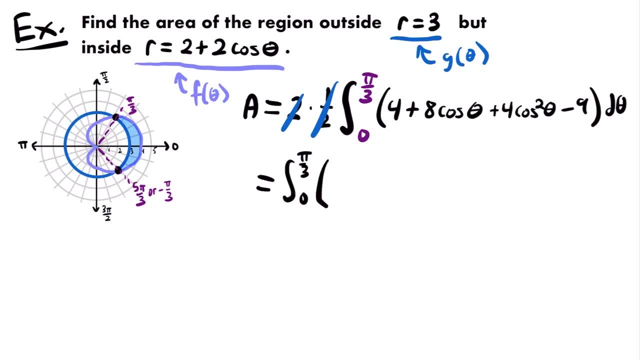 need to first rewrite it using a trig identity, And so I'm going to take care of that right away, And if you're not familiar with that method, feel free to check out my lesson on solving trigonometric integrals, which is the main skill that we're going to be using. 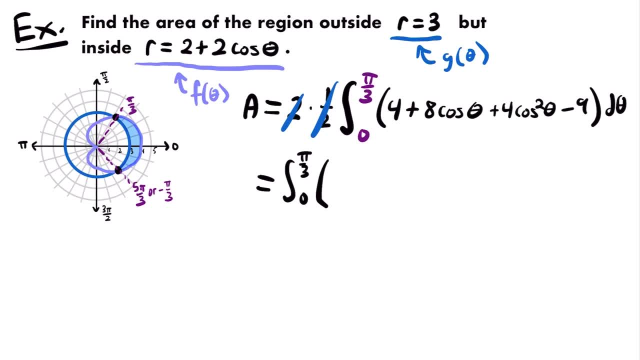 when solving these integrals to calculate the area between polar curves. Alright, so here's what we'll have. I'll write the negative five at the end, the negative five that we get from four and negative nine being combined. So we'll start with eight times cosine theta. 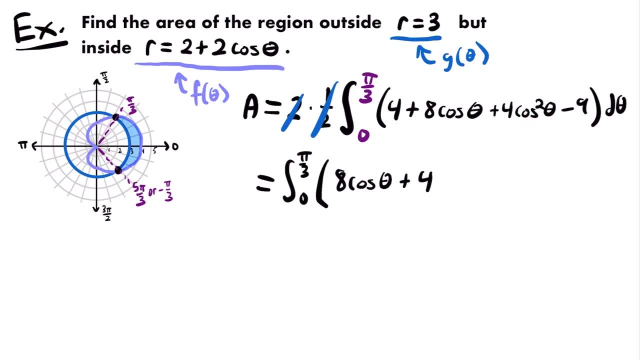 And write cosine squared theta using the following trig identity: We're going to multiply by one half times one plus cosine of two theta. alright, One half times one plus cosine of two theta is the same as cosine squared theta. They are equal to each other. 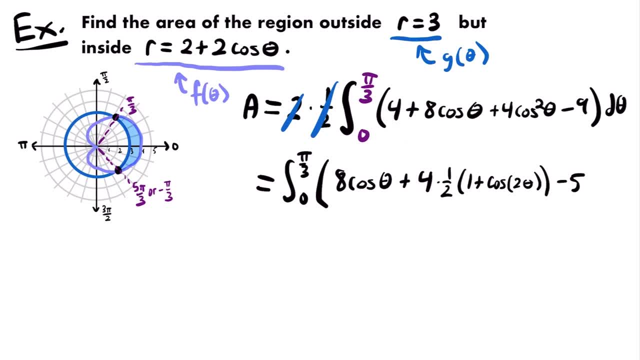 And then we'll have minus five. That comes from adding four and negative nine. okay, Now, next, I'm gonna simplify this a little bit. Four times one half is two, so we'll have two times this quantity, So we'll have two times one and then two times cosine of two theta. 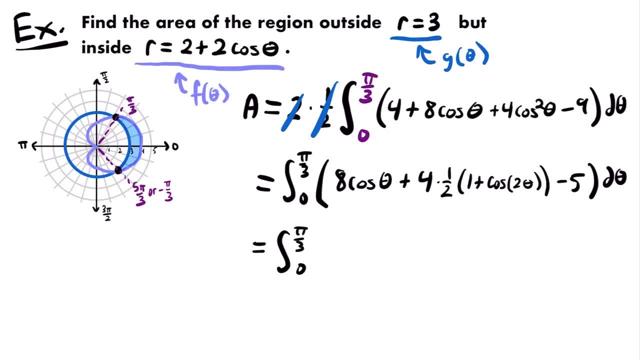 So this is equal to the integral from zero to pi divided by three of eight times cosine theta plus two plus two times cosine of two theta minus five d theta. And now we have two more constants that we can combine. two and negative five will become. 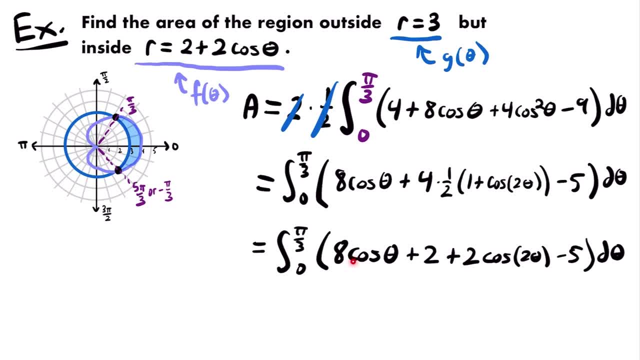 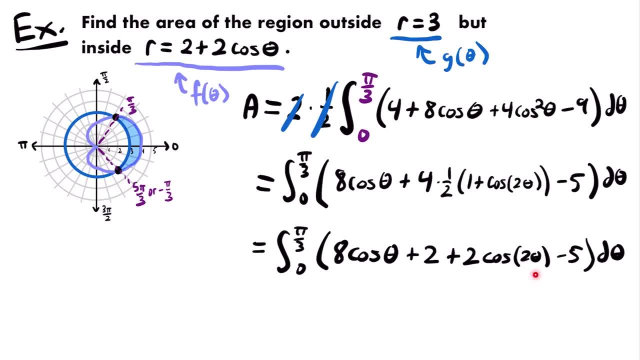 u substitution, And so what I'm going to do is now split up this integral into three integrals: One for this term, one for our constants and one for two times cosine of two theta. That way, we can work on integrating each of them individually with the different rules. 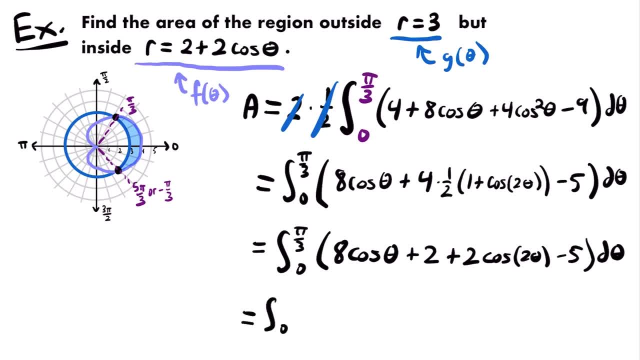 that they require. So we'll have that. this is equal to the integral from zero to pi divided by three of eight times cosine theta d theta, plus the integral from zero to pi, So pi divided by three of two times cosine of two theta d theta. 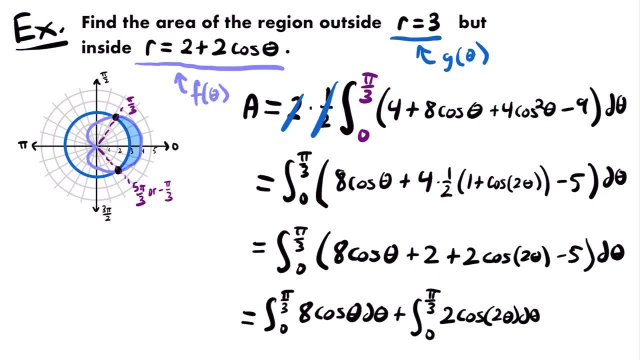 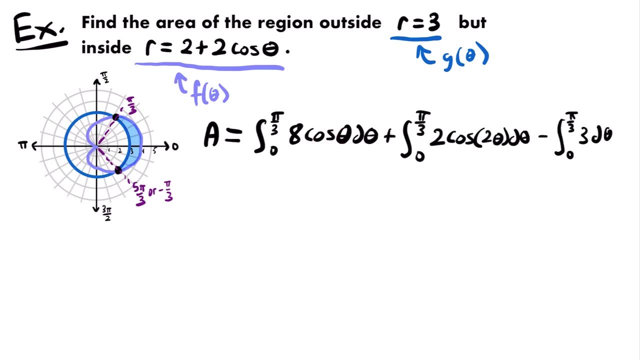 And then, finally, we're going to have two and negative five combined, That's negative three. So we'll have minus the integral from zero to pi divided by three of three d theta. Okay, So now, if we work on integrating each of these integrals, the integral of cosine theta will 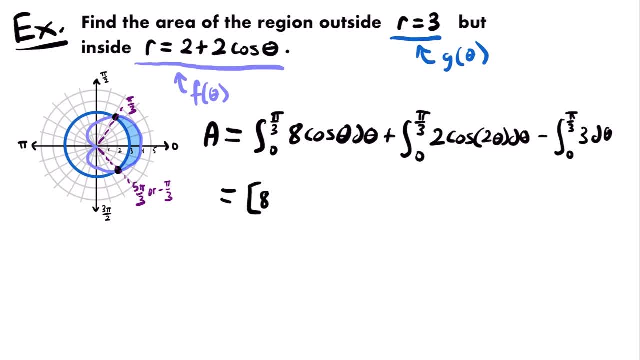 be sine theta. So this is equal to eight times sine theta, evaluated from zero to pi divided by three. Then we'll add that to this integral. but now I'm going to use u substitution. You need to set u equal to this: inside function of cosine. 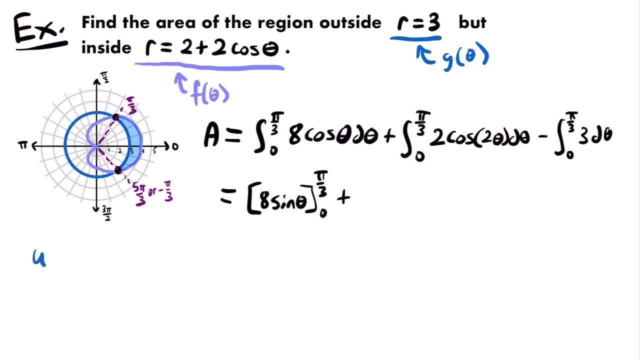 So we'll have: u is equal to two theta. I'll do that on the side here. U is equal to two theta, which means that du d theta, the derivative of u with respect to theta, will be two, And that gives us that du is equal to two times d theta if we multiply both sides by. 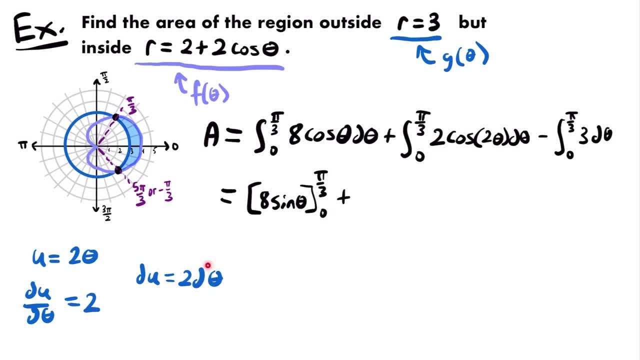 d theta, And so if du is equal to two times d theta, we need to be able to find that within our integral, And we can. we have two nd theta right here, So we can replace that with du. So if we rewrite our integral in terms of u, we'll have plus the integral from zero. 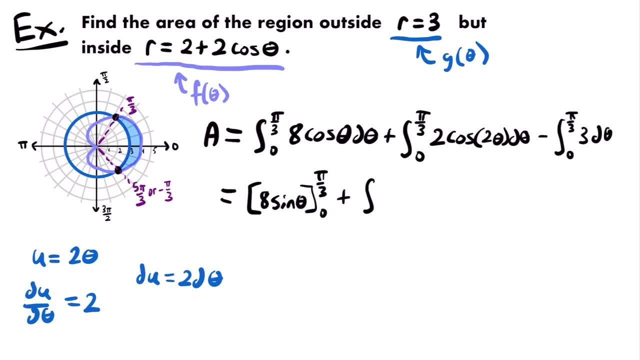 to pi divided by three. but those are bounds of theta. I want to rewrite them in terms of u, So we'll work on that in just a second. We'll come back to that, but then we'll have cosine of u times du. 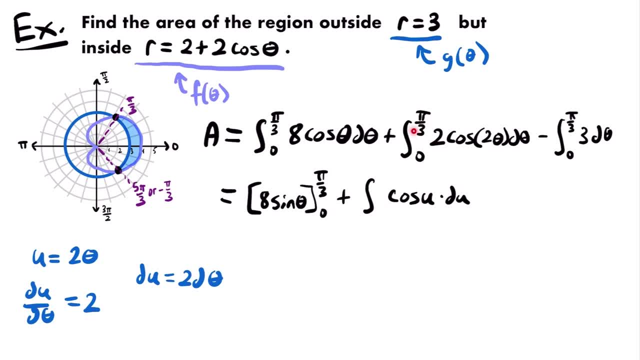 All right, now let's work on those bounds of integration. These are values of theta. They need to be in terms of u, So we'll plug these values of theta into what we set u equal to. So if theta is zero, we'll have zero times two, which is zero. 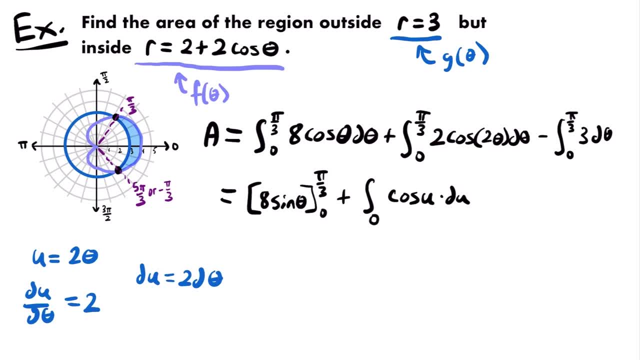 So the lower bound will still be zero. That's our lower bound in terms of u. And then for the upper bound, pi divided by three. if that's theta, you have two times pi divided by three, which will be two pi divided by three. 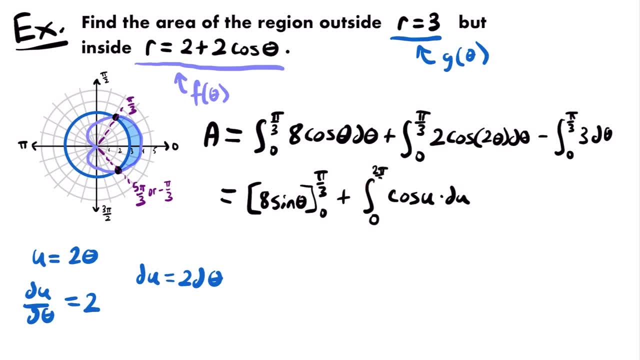 So that's the new upper bound in terms of? u. We'll have two pi divided by three, All right, and then we will subtract the integral of three, which is going to be three theta, And that is evaluated from zero to pi divided by three. 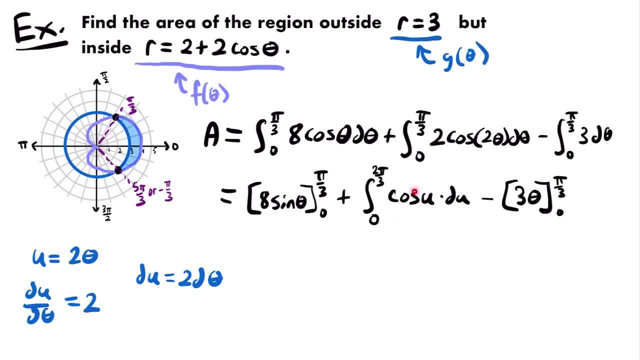 All right. so now this integral right here is entirely in terms of u, So we don't need to worry about going back to terms of theta. We can just integrate and evaluate in terms of u. All right now, if we evaluate eight times sine theta at pi divided by three and subtract, 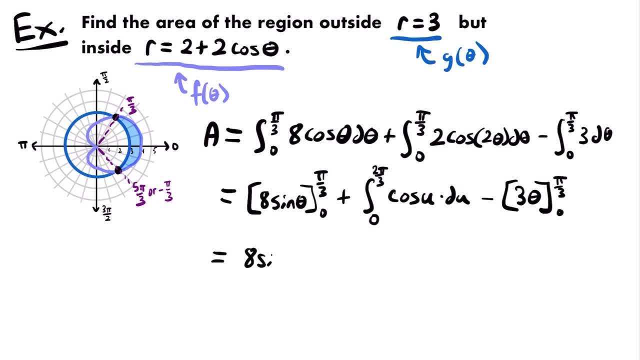 the evaluation at zero, this will be equal to eight times sine of pi divided by three. And then you'd have eight times sine of zero. but sine of zero is zero, so we'd just be subtracting zero. So I'm not going to bother to write that here to save some space. 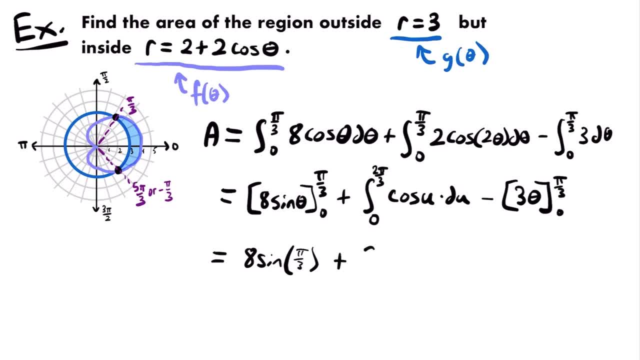 And then the integral of cosine u will be sine u, so we'll have plus sine u, evaluated from zero to two pi divided by three minus three times pi divided by three minus zero. All right, we evaluate three theta at pi divided by three and subtract the evaluation at zero. 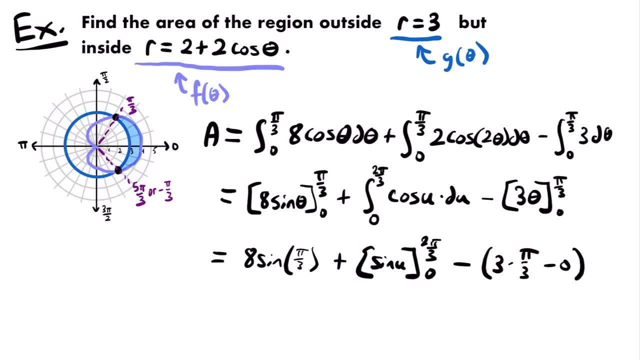 And so three times pi divided by three, we have right here. and then three times zero is zero, so we're subtracting zero. Okay Now, sine of pi divided by three, that's equal to the square root of three divided by two. 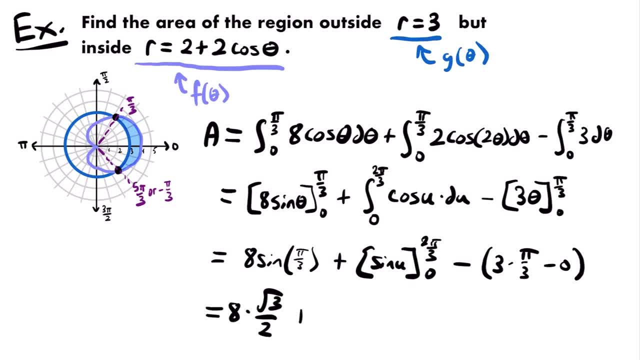 So this is equal to eight times the square root of three divided by two, And we'll add that to sine evaluated at two pi divided by three minus sine of zero. Sine of zero is just zero, so we don't have to worry about that. 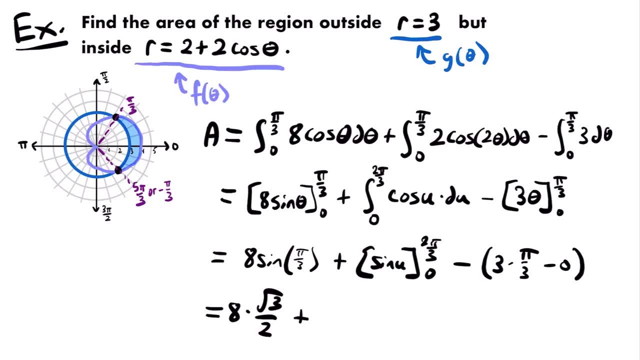 But sine of two pi divided by three is also the square root of three divided by two. So we'll have the square root of three divided by two, and then we are subtracting three times pi divided by three. Those threes will cancel out. 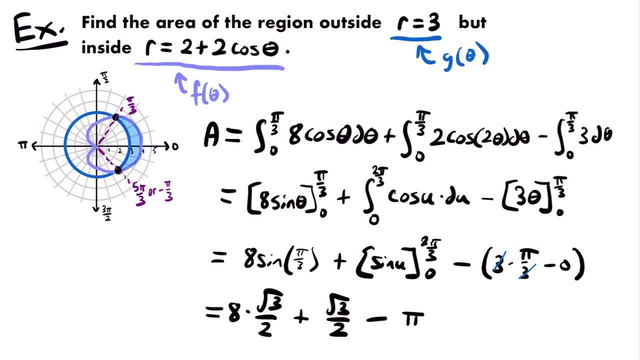 leave us with pi, And so we are subtracting pi. Okay, now we have 8 times the square root of 3 divided by 2, or you could rewrite that and just have 8 times the square root of 3 divided by 2.. And so, if you have 8 square roots of 3 divided by 2, plus 1 square root, 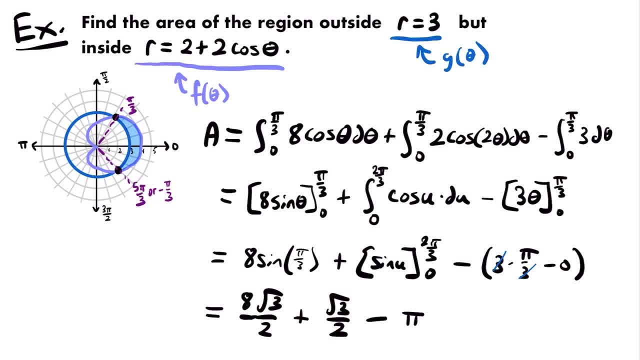 of 3 divided by 2, you'll have 9 square roots of 3 divided by 2.. So this is equal to 9 square roots of 3 divided by 2 minus pi. And that right. there is the answer in its simplest. 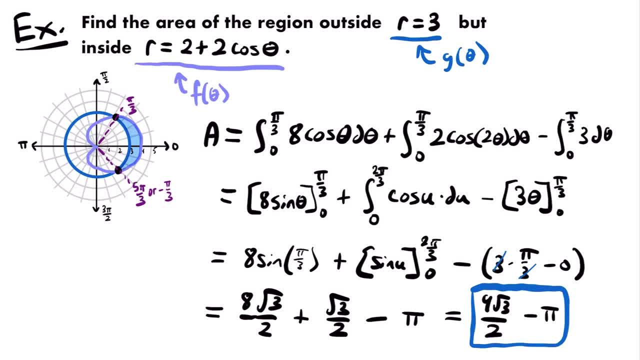 form. This is the area of this region that lies between these two polar curves. Okay, and so that's the general process that we can use for calculating area between polar curves. And so, before we look at our next example, which will be a little bit more complicated, 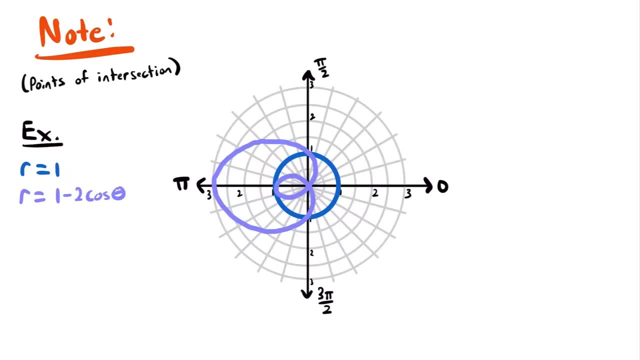 I want to quick make you aware of something interesting. I wanted to take a little side trip here and make a note about points of intersection when it comes to two polar curves. Here I have a quick little example of two polar curves. We have r equals 1 and 2 are poles on theötary, And we have r equals 1- mom and 2 is the square. 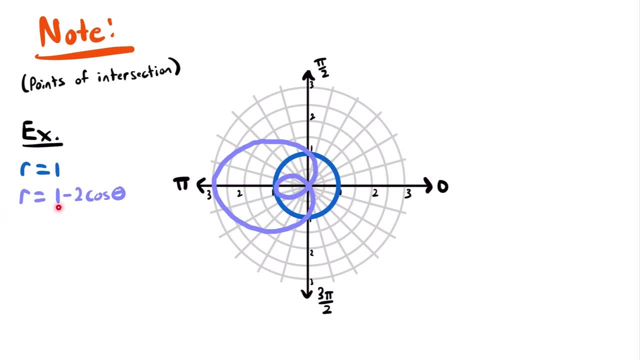 And we have: r equals 1 and 2 is the square, And the square is 2 and 2.. So this is the area one, that is, this circle right here, and r equals one minus two times cosine theta, which is this lima sun with an inner loop. 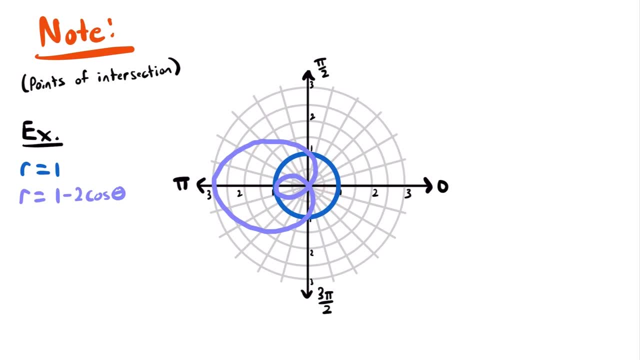 You can see visually from this graph here that these two polar curves intersect at three different places. They intersect right here, they intersect down here and they also intersect right here where we have that inner loop for this lima sun. All right, so we can see visually. 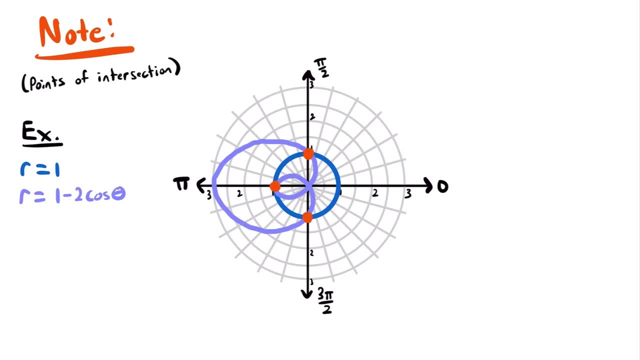 by graphing these two polar equations that we have three points of intersection. but if we were to try to find the angles of theta for those points of intersection by setting our two polar equations equal to each other, something interesting is going to happen. So let's do that on the side here. 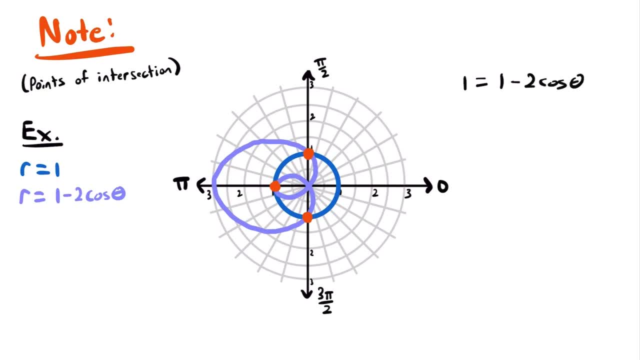 We'll have. one is equal to one minus two times cosine theta. I'm just setting this polar equation equal to this one. So we have one and that's equal to one minus two times cosine theta. Let's solve for theta here and see what happens. 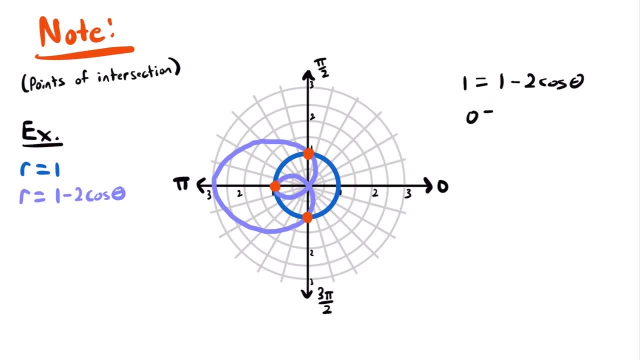 If we subtract one from both sides of the equation, we'll have zero is equal to negative two times cosine theta, and then dividing both sides by negative two will give you zero is equal to cosine theta, and we know that cosine theta is equal to zero. 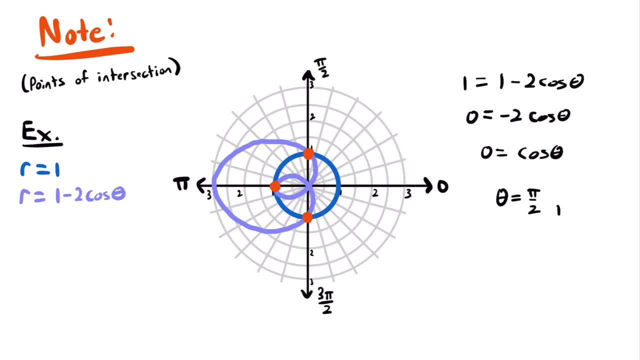 when theta is equal to pi divided by two and three pi divided by two. So what we found here are two angles of theta where our curves will intersect at an angle of pi divided by two. That's this angle right here, and so that will correspond to this point of intersection. 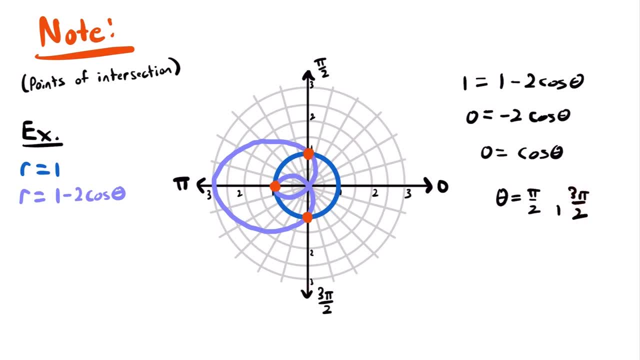 and then we have three pi divided by two, which is this angle right here, and so that will correspond to this point of intersection. But notice that we don't have an angle for pi right. Our two polar curves intersect at this point. 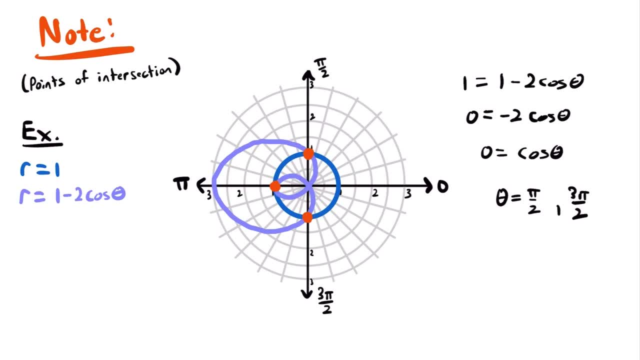 but we didn't find that angle of theta by setting our curves equal to each other, And so why is this the case? Why does this happen? How come we didn't get theta equals pi as one of our angles where we have a point of intersection? 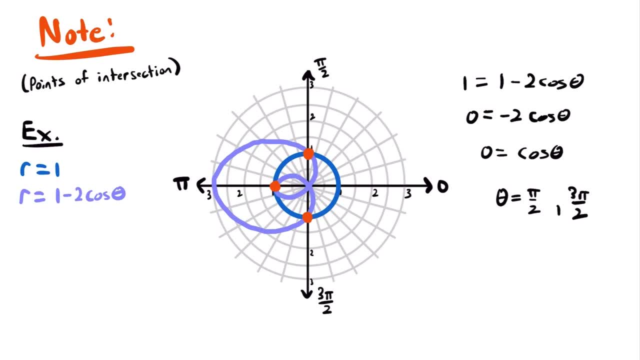 Well, what's actually going on here for these two curves is that at these two points of intersection, where we found these angles, those two points occur at the same angle for both curves. When you draw or trace your polar curves, starting at the angle of zero, 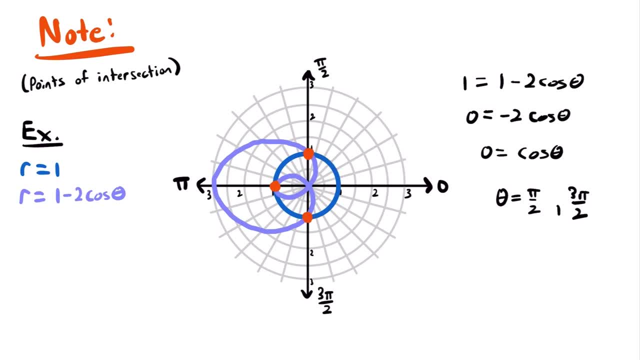 they're both at those points, at the same angle. They're both at those two points, at pi divided by two and three pi divided by two, But at this point these two polar graphs are at completely different angles. All right, specifically that point of intersection. 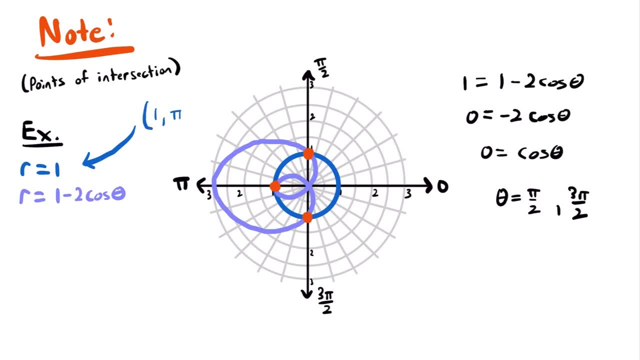 for r equals one is at the point one comma pi, but the point for this polar equation r equals one minus two times cosine theta is negative one comma zero. These are two polar coordinates that represent the same point. This goes back to one of my earlier videos. 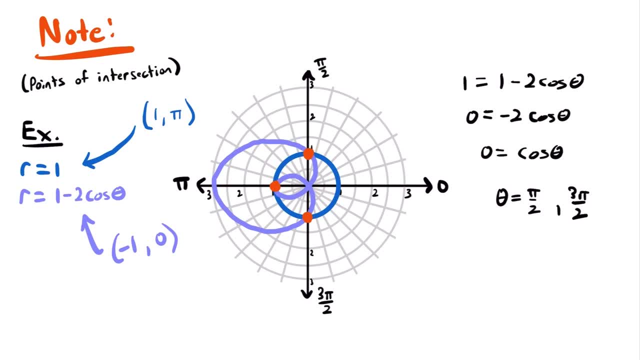 where I talked about polar coordinates and how you can have different sets of polar coordinates that represent the same point in the polar coordinate system. These two sets of polar coordinates have completely different angles. We have pi and zero, but we're still at the same point. 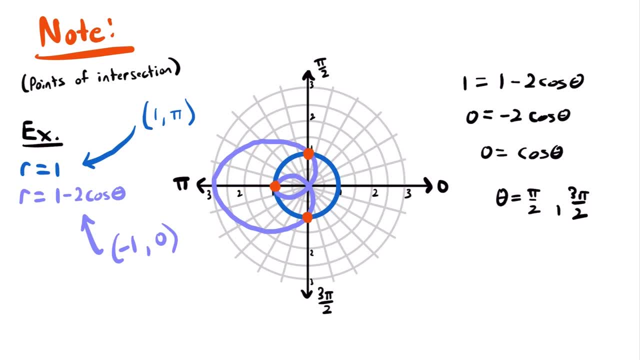 We still have a point of intersection between these two polar curves And you can see that if you were to plot these two sets of polar coordinates, An angle of pi will take you to this angle right here, and a radius of one takes you to this point right here. 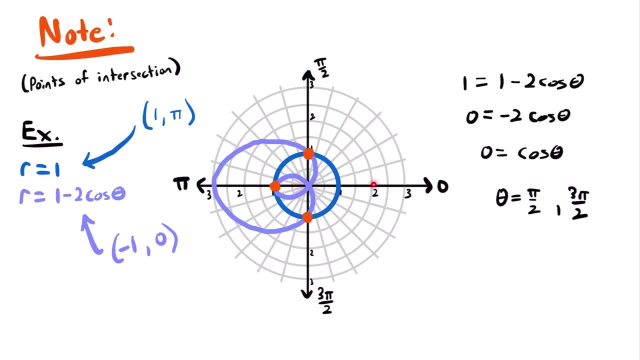 And then for this coordinate point, our angle is zero, so we're going to be along this angle right here, but our radius is negative one, so we would measure out to a radius of one, but since it's negative, we have to reflect it. 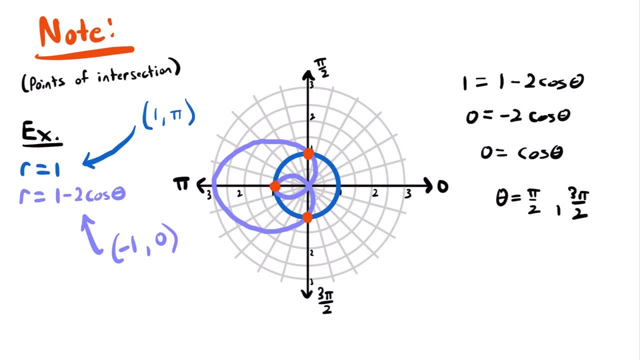 to the other side. so we're also at that point, All right, and so the reason I point this out, the reason why it's important to see this, is because it gives you all the more reason to graph your polar curves When you want to calculate the area. 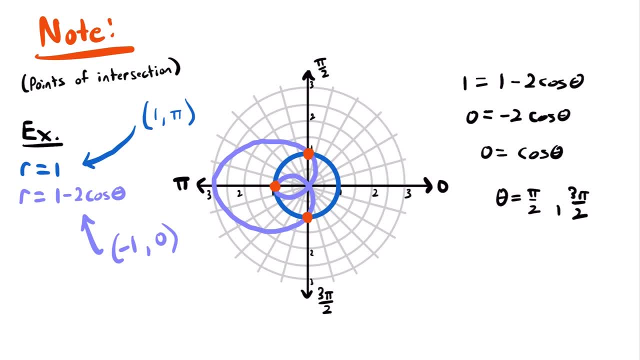 between two polar curves and you need to determine points of intersection so that you know what two angles to integrate between. you need to graph your curves. If you don't, you might miss out on some points of intersection because sometimes they're not going to occur. 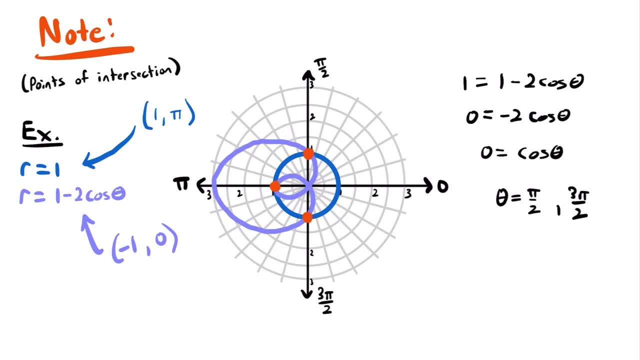 at the same angle. Okay, and then one more thing to keep in mind: Remember that if you have a pair of polar coordinates of zero and then any angle, theta that is going to represent the same point. right, If your radius is zero, you're guaranteed to be at the pole. 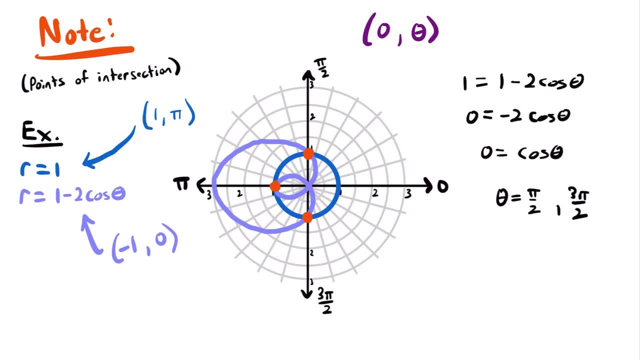 because that is where the radius is zero, And so if you have a radius of zero, any angle theta will take you to that same point, And so, once again, you could have two polar graphs with two different pairs of polar coordinates. Let's say we had zero pi and then zero pi divided by six. 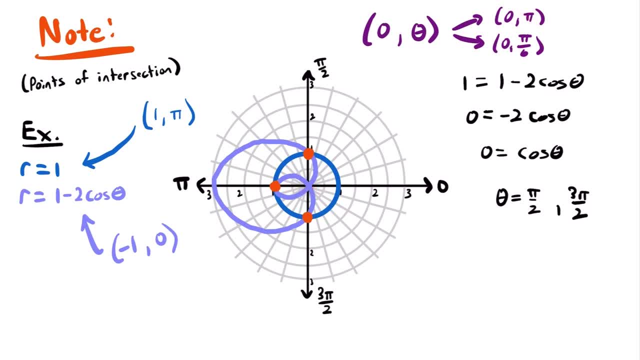 These two polar coordinates would represent the same point at the pole. These two points have different angles, but they still represent the same point. So if you had two polar curves that intersected at the pole or at the origin, you won't always be able to detect that. 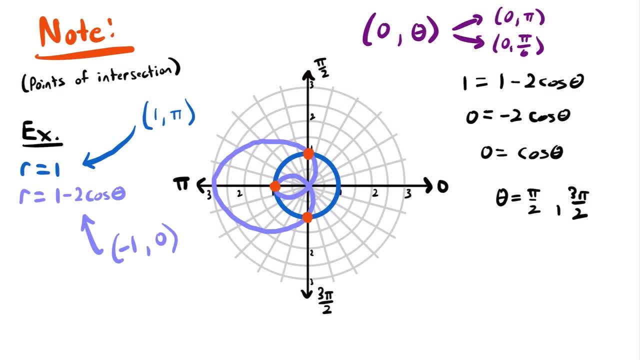 from setting your polar equations equal to each other. Okay and so, while you could see that visually, you could always see by graphing your polar equations if they intersect at the pole. it could also be helpful for you to check that manually by setting each of your polar equations equal to zero. 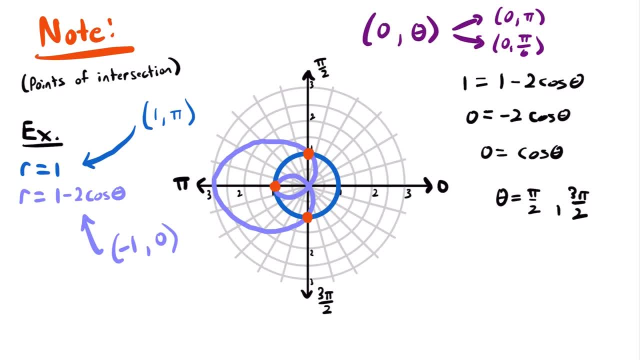 and solving for theta. Okay, so that's just something to keep in mind as well, But in the end, the big takeaway here is: always graph your polar equations when you want to calculate the area of a region between two curves. If you don't graph your region, 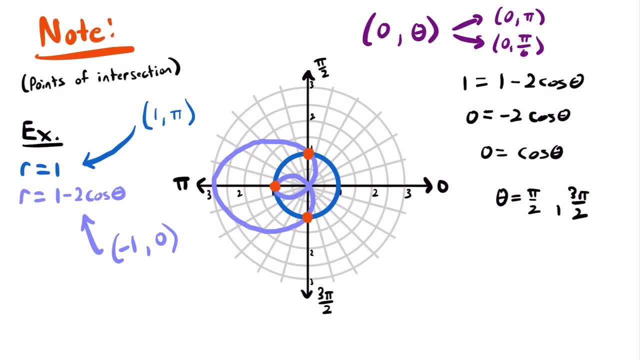 you're probably going to make a mistake, because you might not identify some points of intersection that you would have been able to identify had you graphed your polar equations. Okay and so with that, let's take a look at one more example for this video. 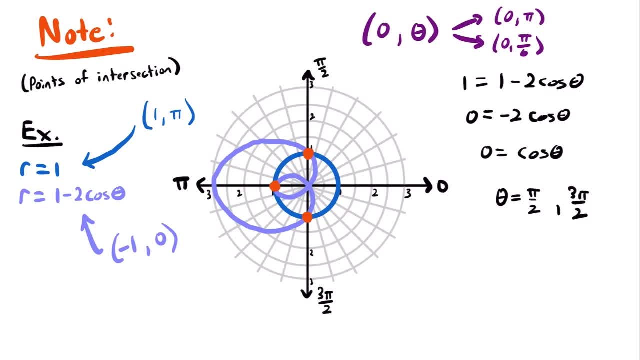 which will demonstrate one of my earlier points, that sometimes you will have to think a little bit intuitively when setting up your definite integral to calculate the area bounded by two polar curves. And so let's take a look at that example next. All right, so here's our last example for this video. 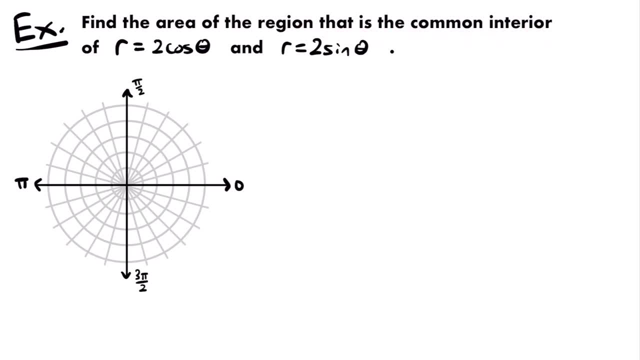 You want to find the area of the region that is, the common interior of. r equals two times cosine theta and r equals two times sine theta. All right now, this is a little bit different than our first example. Whenever a problem asks you to find the common interior, 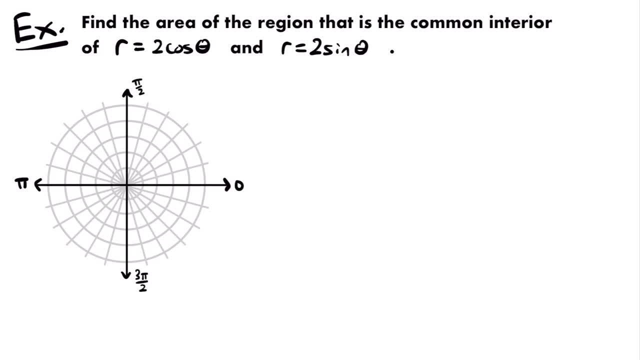 between two polar equations or two polar curves. it's most likely the case that just subtracting the area beneath one curve from the area of the other curve is not going to be how you find the area of that common interior. All right, we're not going to be able to use. 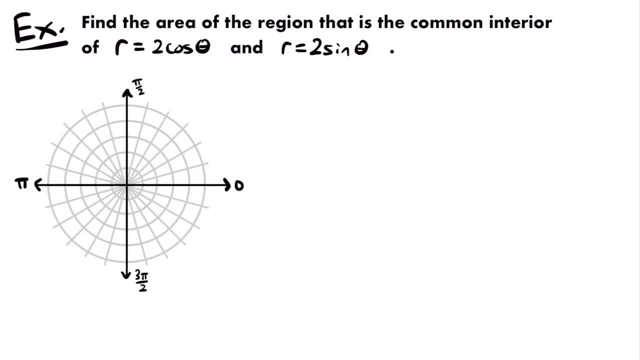 that same formula, or that same definite integral that we found at the beginning of this video, And so let me show you what I mean. Let's graph both of these polar equations and see what this region is, that we want to calculate the area of. 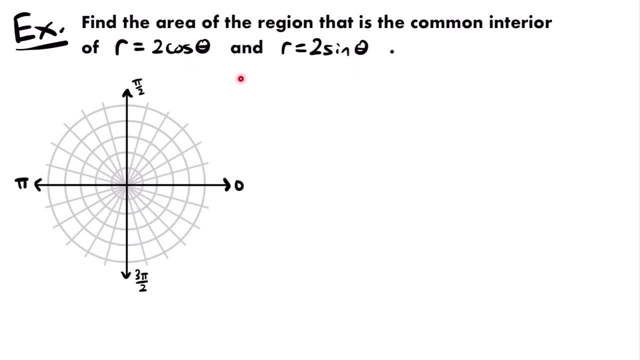 Now, both of these polar equations are basic polar graphs. Both of these equations just represent circles that are not centered at the origin. They're both going to have a diameter of two. That's what the constant is. The constant in front of those two equations tells us: 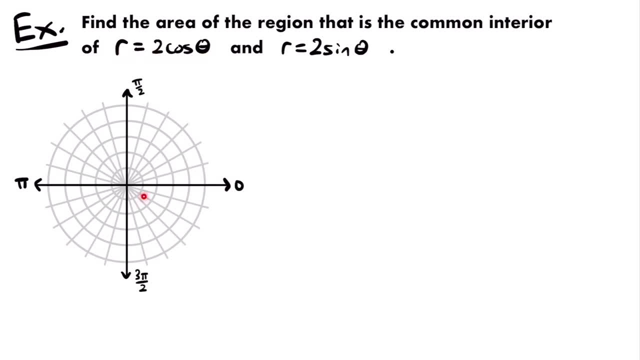 And r equals a constant times cosine theta, will be a circle along the polar axis, along the right side of our vertical axis, given that this constant is positive, and that circle will have a diameter of that constant. So r equals two times cosine theta. 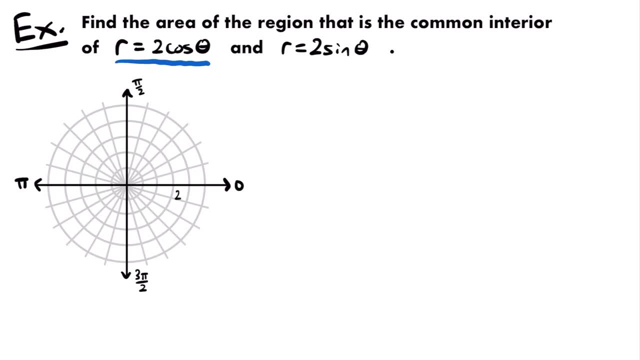 if this circle right here represents a radius of two, that means that the radius of two will be right here, right here and right here, And so then our polar curve will look like this: All right, we have a circle that is split. 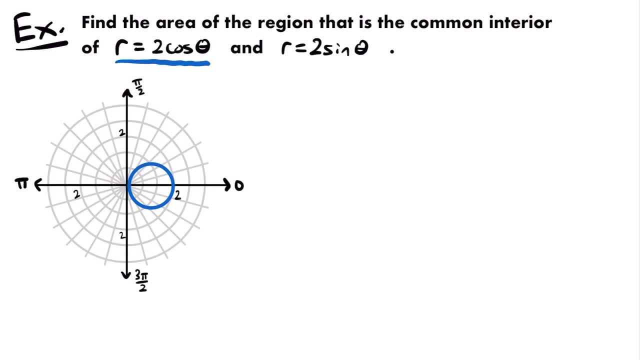 by the polar axis and it's on the right side of the vertical axis, with a diameter of two, All right. and then for r equals two times sine theta. when you have a constant times sine theta, that's going to be a circle that rests above the polar axis. 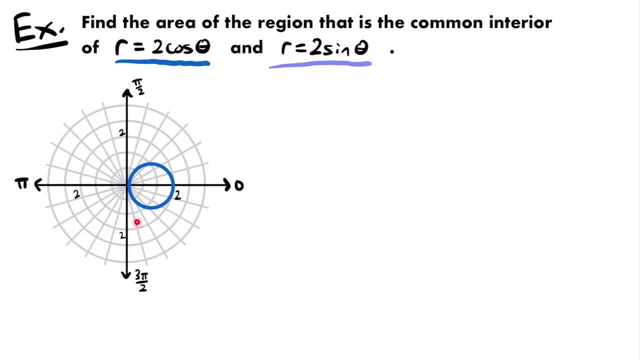 and it's split by the vertical axis. It will be below the polar axis if that constant was negative, but we have positive two, so we're going to have a circle above the polar axis with a diameter of two, And so that circle will look like this: 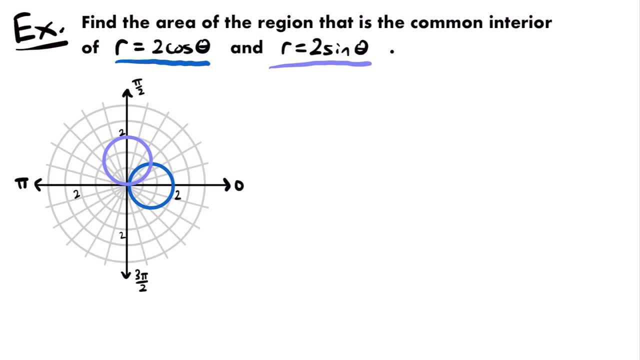 All right, and so now we have both of our polar curves here and we want to find the area of the region that is the common interior of those two polar equations or of those two polar curves. So if you look at our graph here, 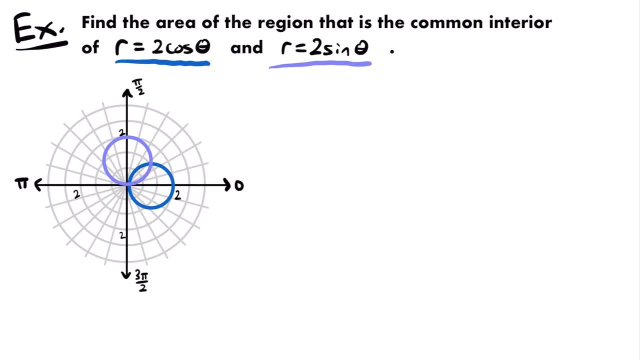 the common interior is this little section right here. If you look at it from an angle, this sort of looks like a Venn diagram. That common interior would be that middle section of the Venn diagram right. You kind of have this overlapping area. 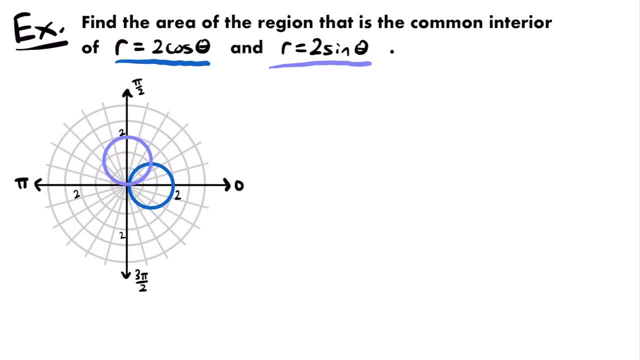 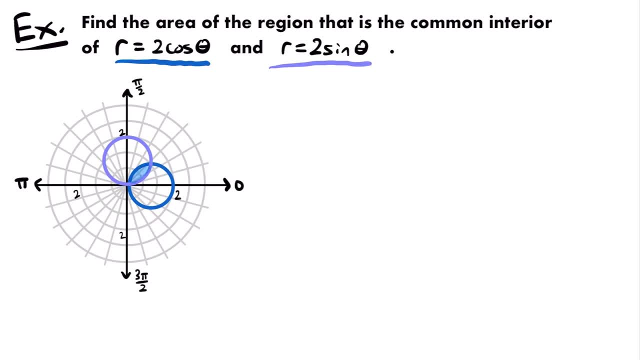 All right, and so now we have two polar curves, And so I'll shade that in. This is the area that we want to calculate, And now the next thing that we should work on determining here are the points of intersection. That's going to help us set up our definite integral. 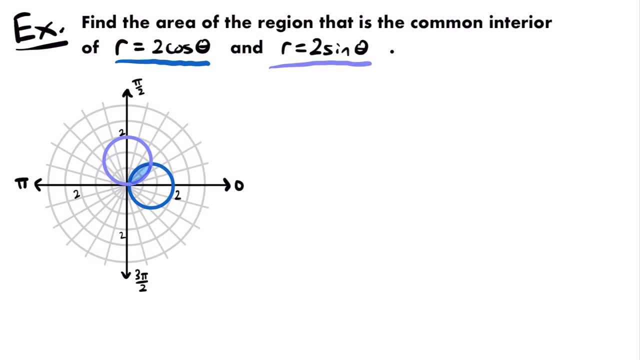 to calculate that area, And so you can see that we have two points of intersection. We have one point right here and then we also have a point right here. But that's just the pole, That's the origin. We don't really need to find that per se. 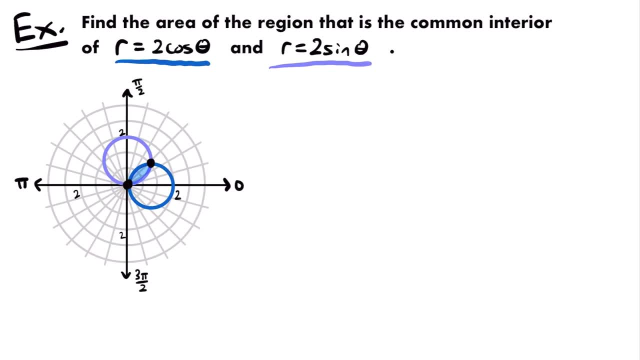 We can already see that our two curves do meet at the origin. But let's find the angle that corresponds to this point where these two curves intersect. So we'll set our two polar equations equal to each other And we'll have two times cosine theta. 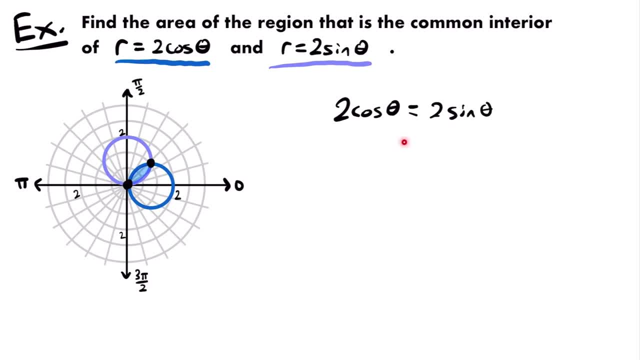 is equal to two times sine theta, And if we divide both sides by two, we'll have cosine theta equal to sine theta. Now for angles from 0 to 2 pi, cosine and sine are only equal to each other at two angles. 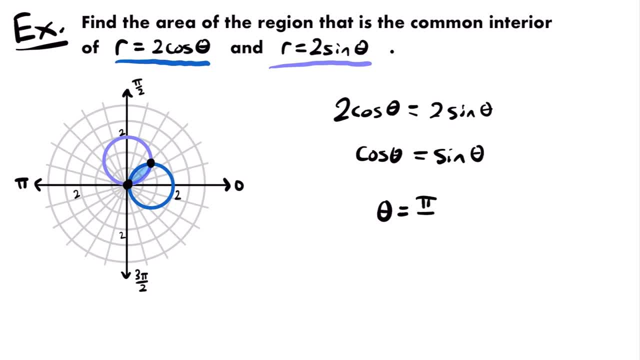 They both will give you the same value for angles of pi divided by 4 and 5 pi divided by 4.. Now, if you look at our graph here, pi divided by 4 is the only one that applies in this scenario. An angle of pi divided by 4 will be halfway in between an angle of 0 and pi divided by. 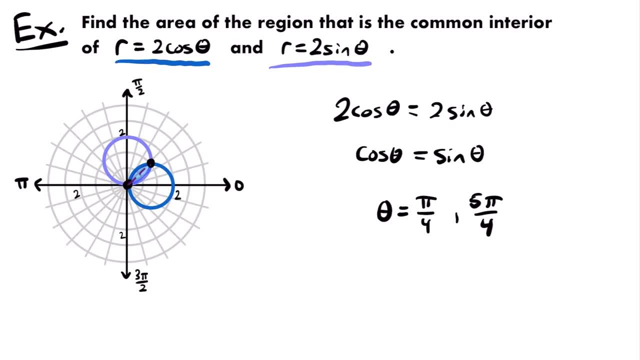 2. So that is this angle right here. So I'll plot that here. That's our angle of pi divided by 4.. And then we can just ignore 5 pi divided by 4, because that's not going to apply to this. 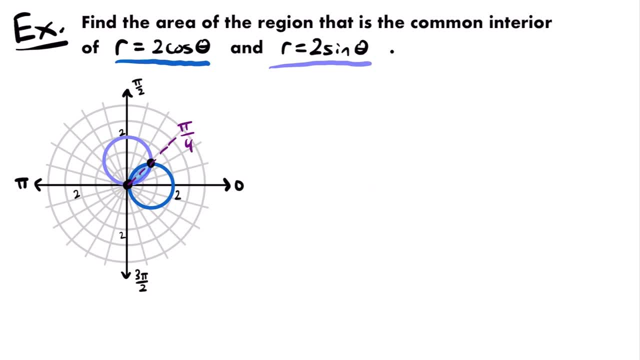 graph. OK, So now we know that this point of intersection right here is at an angle of pi divided by 4. And we can use that to help us set up our definite integral to calculate this area. Now, what I want you to notice about this area, however, is it's a little bit different than 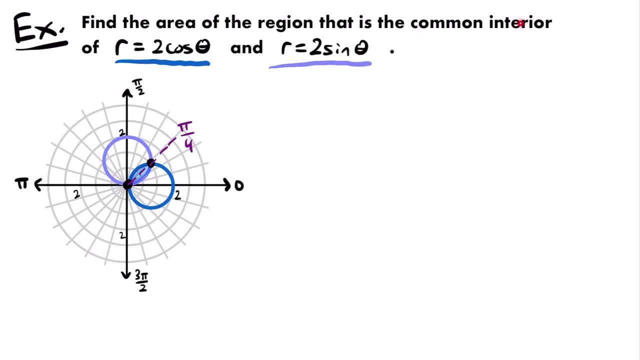 our first example. This area is a common interior. It's not really the area between two curves. it is the area shared by two curves, And so this is a little bit different. We're not going to be able to calculate this the same way. 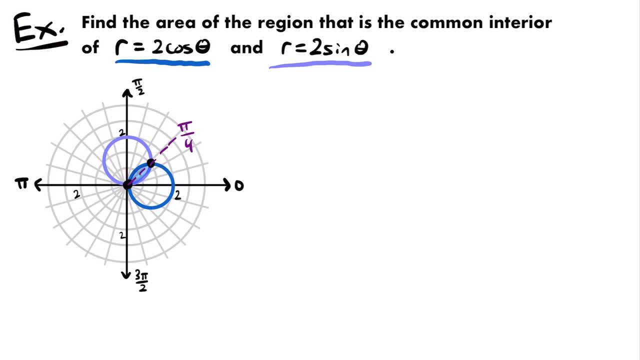 We can't just subtract the area beneath one curve from the area of the other curve. All right, And let me show you what I mean. If we were to look at this area up close, individually, for each circle, If I were to draw two graphs here, one for each circle, 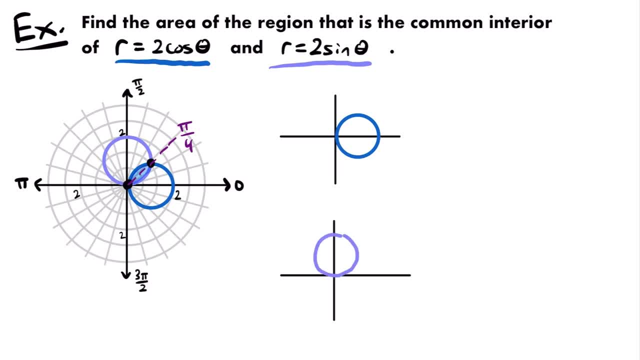 Here's our circle for 2 times cosine theta and here's our circle for 2 times sine theta. This area would be split in half. Half of this area is contained by this circle and the other half of this area is contained by this circle. 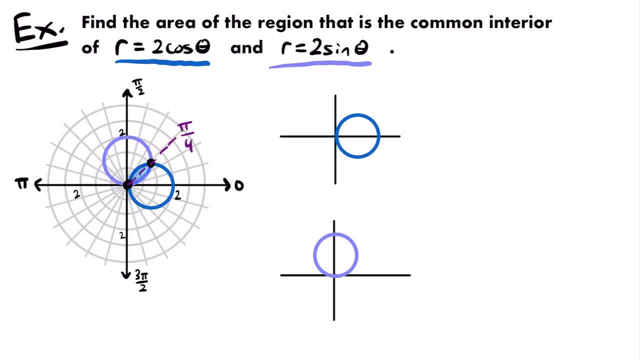 Right If I were to draw in that angle of pi divided by 4 in each of these graphs. watch what happens. Here's that angle of pi divided by 4.. It's right between an angle of 0 and pi divided by 2, and we'll draw the same thing down here. 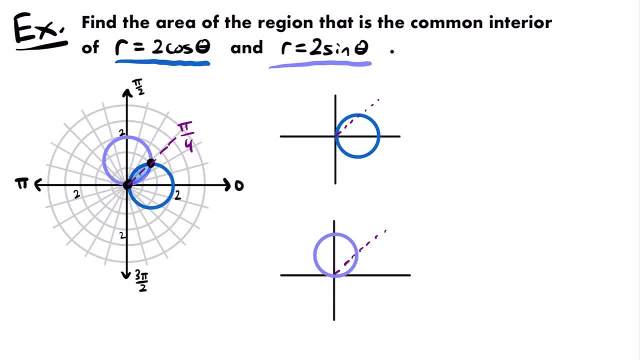 There's our angle of pi divided by 4. You can see that only half of that area rests in each of these circles. We have half of the area right here and half of the area right here, And both of those halves of the area are only contained within one curve. 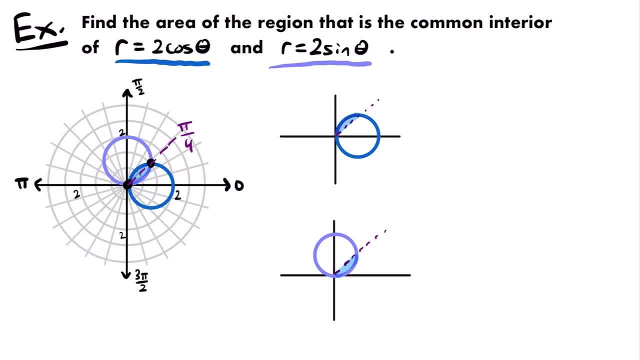 Right. This section is the area beneath this circle. It's not between two curves, It's just within itself. And the same thing applies to this little bit of area: It's not between two curves, It's just within one curve: This circle. 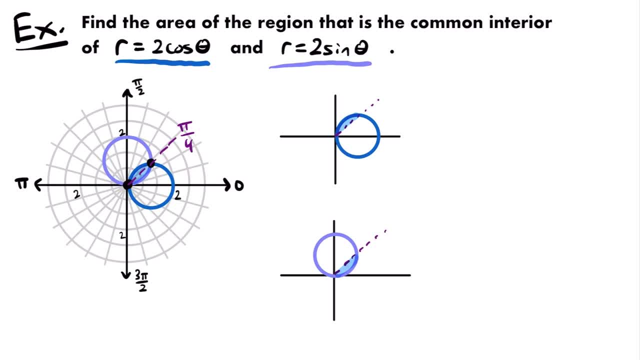 So setting up a definite integral to calculate this area is going to be a little bit tricky. One way that we could go about it is set up a definite integral to calculate this area and then add it to a definite integral that calculates this area. We could do it in two parts. 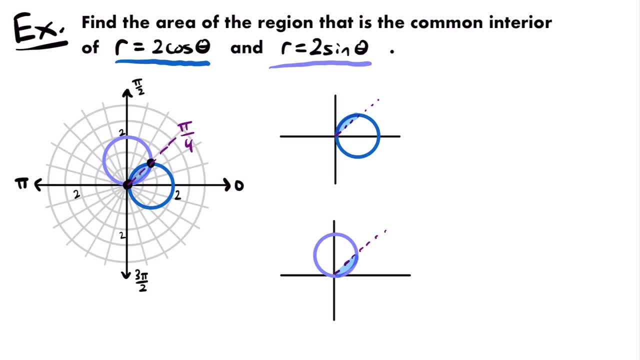 However, this area that we're trying to calculate is going to be a symmetric area. It is split evenly by that angle of pi divided by 4. And so this half of the area is the same as this half. So what we can do is make use of symmetry and only calculate the area of one half of. 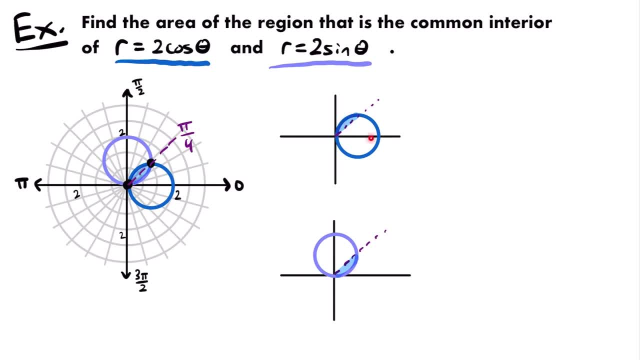 that area and then just multiply it by two. So we can choose one of these two areas within one curve, calculate that area and then multiply it by two, And I'm going to choose this area right here. This one will be easier because this area beneath this circle or beneath this curve. 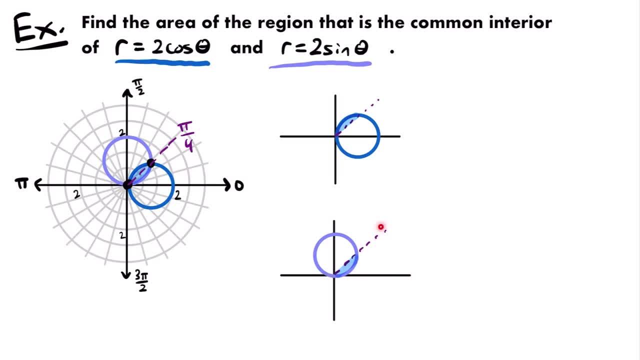 Is going to rest between this angle of zero and this angle of pi divided by four. right From this angle to this angle, will be that half of this region, The upper half, this half right here that rests between pi divided by four and pi divided 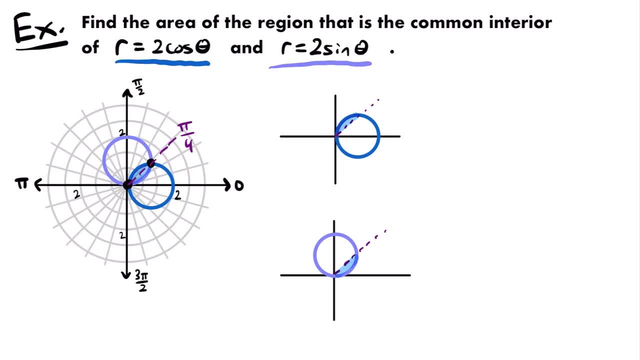 by two, which would be much more complicated to work with as bounds of integration. So what I'll do is set up an integral for the area of this half of that area. All right, So we're just going to be setting up a definite integral to calculate the area beneath one. 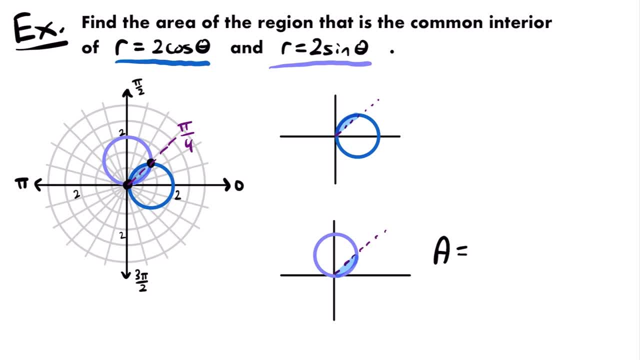 curve, just like if we were calculating the area under one polar curve in the past. And so we'll have one half times the integral from zero to pi divided by four, And then we're going to have r squared, where r is the polar equation for this circle. 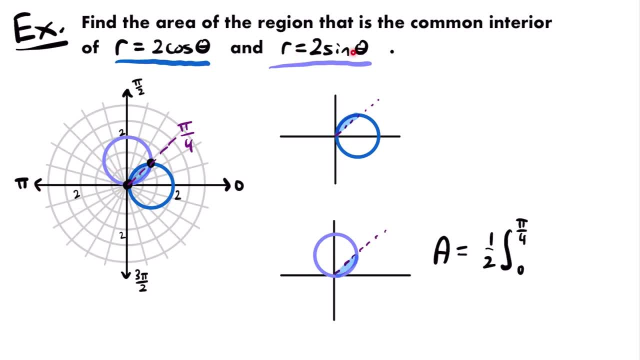 And this circle that is above the polar axis is represented by this polar equation. So we will have two times sine theta squared and then times d theta. All right, So this right here represents the area of this half. So if we want to calculate the area of the whole region, we just then have to multiply. 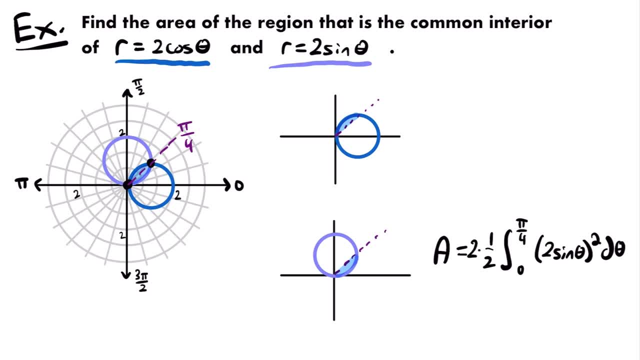 this integral by two, So we'll have two times, one half times, this integral. Okay, So now let's work on solving this integral to calculate the area of this region shared by these two circles, And so let's work on simplifying this. 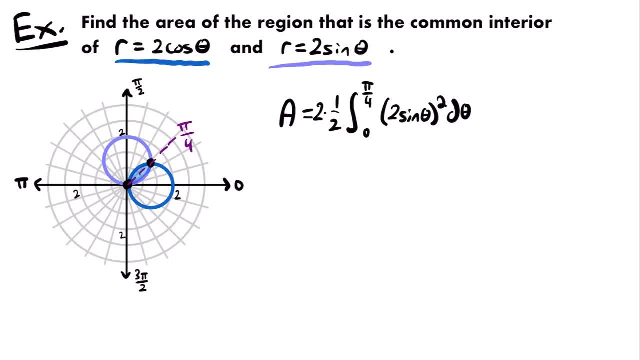 The first thing that I notice is that two times one half is just equal to one, So we can cross those out, and then we can square two times sine theta, So we'll have that this is equal to the integral from zero to pi divided by four of four times. 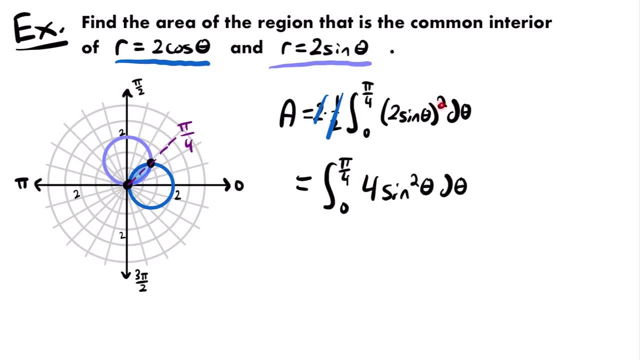 sine squared theta, d theta. All right, Two squared is four, and sine theta squared is sine squared theta, And so now we have a trigonometric integral here that we can solve. In order to solve an integral with sine squared theta, we need to rewrite it using a specific 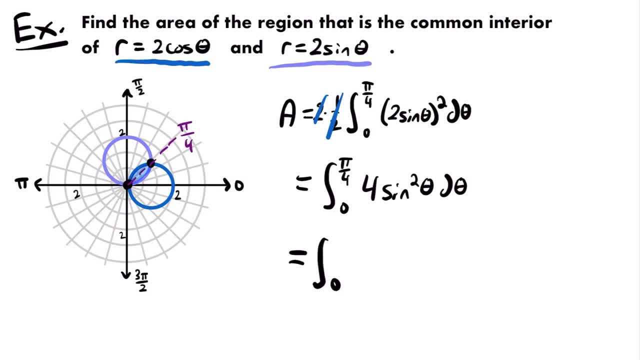 trig identity, And that will look like this: We'll have the integral from zero to pi divided by four of four times the identity for sine squared theta. And that identity looks like this: We'll have one half times one minus cosine of two theta d theta. 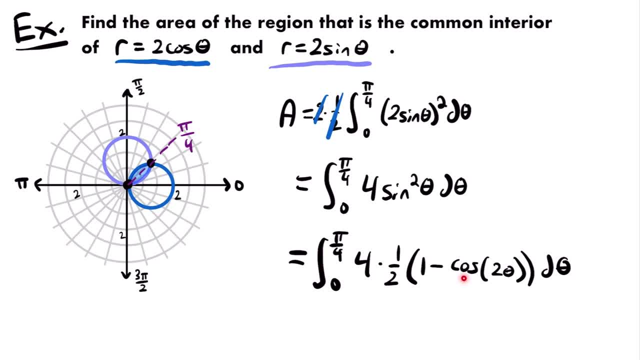 All right. So one half times the quantity one minus cosine of two theta is the same as sine squared theta, They are equal to each other. All right. Now, if we simplify four times one half is two, And so we'll have two times both of these terms. 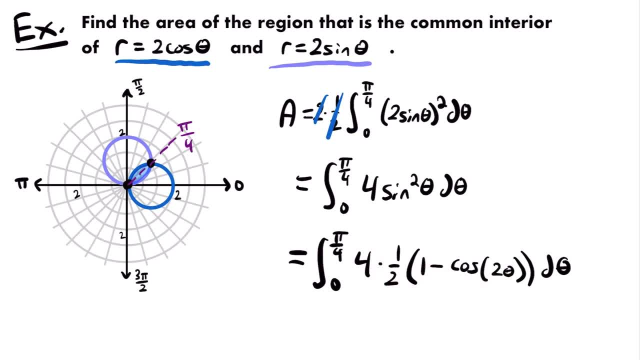 So we'll have two times one, which is two, And then two times the negative cosine of two theta. So we'll have minus two cosine of two theta. So this is equal to the integral from zero to pi divided by four of two minus two times. 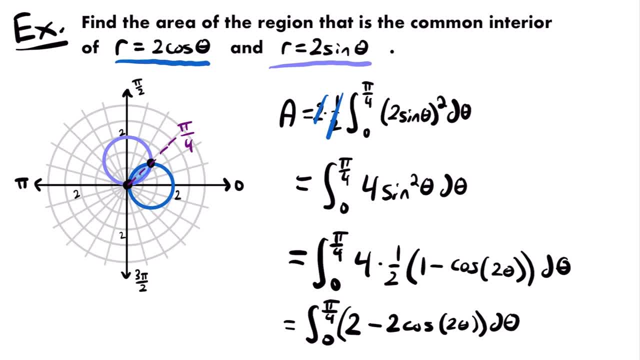 cosine of two theta d theta. Okay, And so now what we can do is split this integral into two integrals: one for this constant term and then one for this term, where we will need to use u substitution. All right, So let's work on splitting this integral up into two integrals. 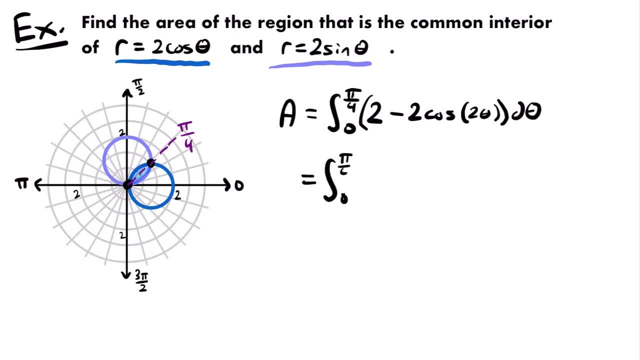 The area is equal to the integral from zero to pi divided by four of two d theta. All right, So we have u theta minus the integral from zero to pi divided by four of two cosine of two theta d theta. Now, if we use u substitution, we'll set u equal to that inside function of two theta. 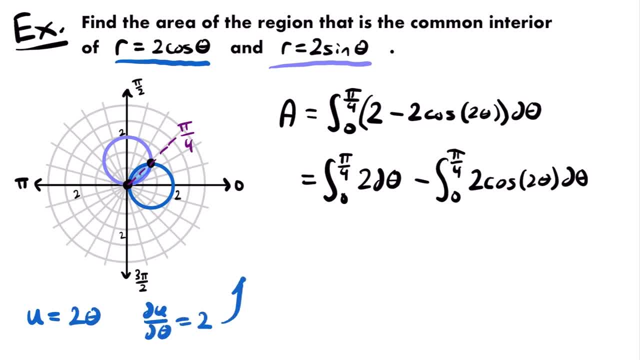 which means that du d theta is equal to two. which means that du is equal to two d theta Right. We multiply both sides by d theta to solve for du. And just a reminder that du d theta is the derivative of u with respect to theta. 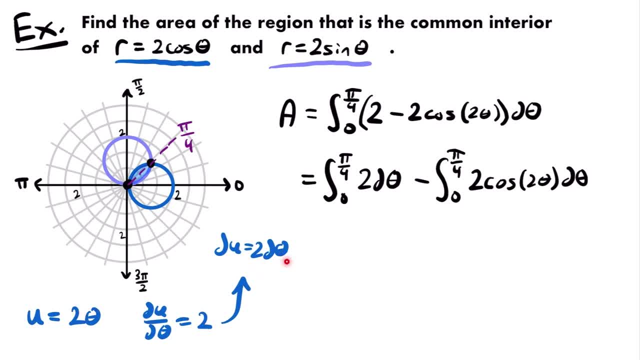 So the derivative of two theta is two, All right, And two d theta is in our integral. So we can replace two and d theta with du, And then we can replace two theta with u, of course, All right. So this is equal to the integral of two d theta. 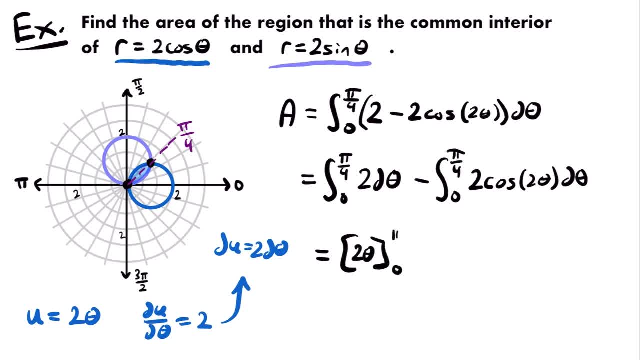 That will be two theta and that will be evaluated from zero to pi divided by four. And then we will subtract the integral of cosine u, du. And now let's rewrite our bounds of integration to also be in terms of u rather than theta. All right, 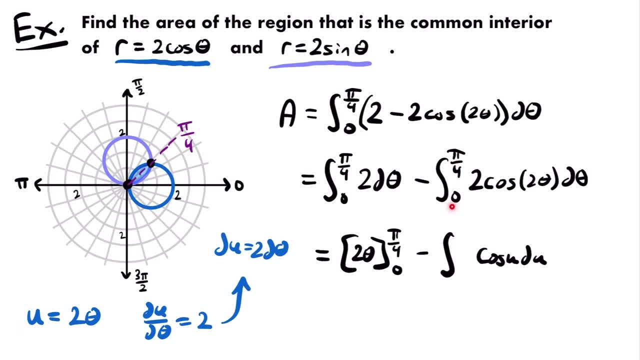 So let's plug our bounds of integration into what we set u equal to. When theta equals zero, we'll have zero times two, which is zero. So u equals zero will be the new lower bound. So we're still going to have zero. 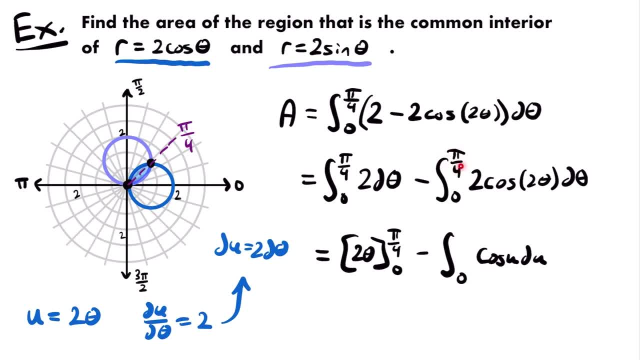 But now that's in terms of u And then the upper bound. we have: theta equals pi divided by four. If we plug that in for theta, we'll have two times pi divided by four, which will be pi divided by two. So the new upper bound in terms of u is pi divided by two. 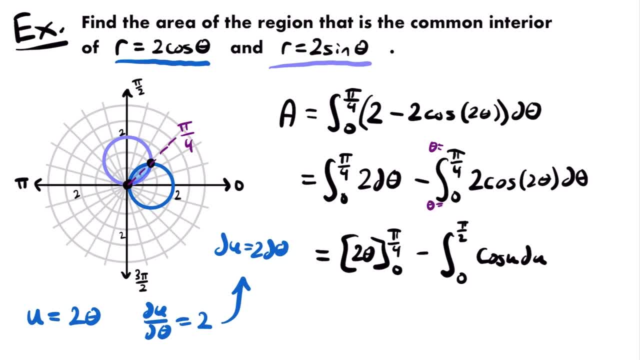 All right, So these were bounds of theta. Just want to make a note of that. And these are bounds of u. Okay, So now, if we simplify two, theta evaluated at pi divided by four will be two times pi divided by four. 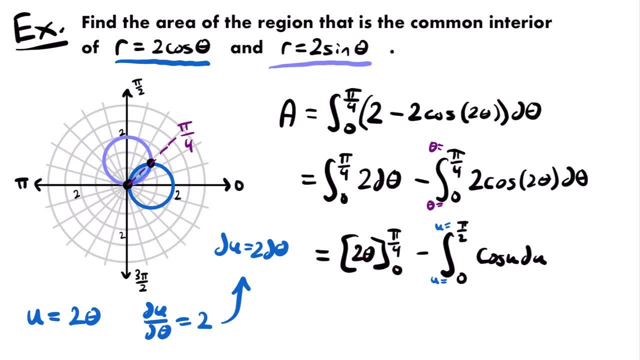 And then we'll be subtracting two times zero, which is just zero. So we're just going to have two times pi divided by four, And then we will subtract this integral, which now is entirely in terms of u, So we don't have to go back into terms of theta. 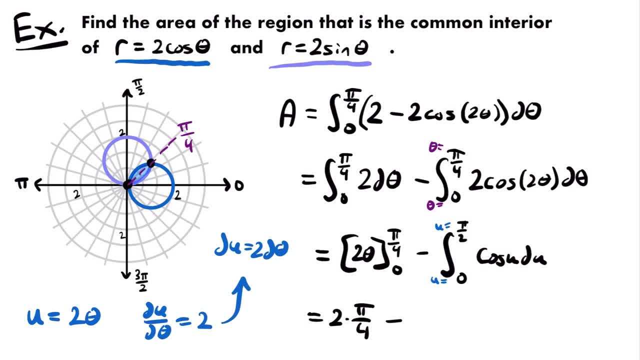 We can just solve it as is. The integral of cosine is sine. So we'll have sine of u Evaluated from zero to pi divided by two, And so now we can simplify what we have here to solve for our area. Okay. 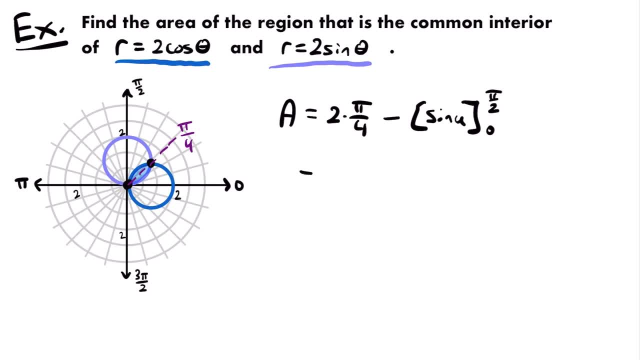 And so two times pi divided by four will be pi divided by two. So this is equal to pi divided by two, minus sine of pi divided by two minus sine of zero. Now, sine of zero is zero. So we're just subtracting zero and sine of pi divided by two is equal to one.